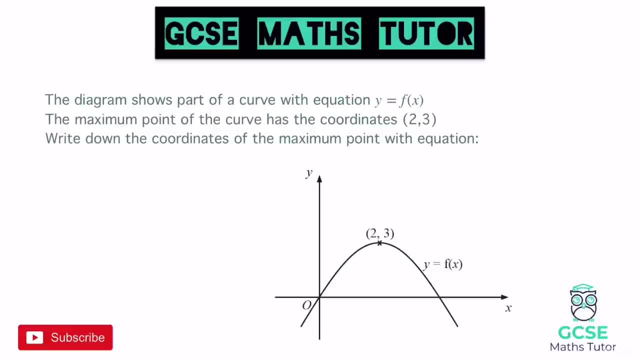 f of x. Okay, so it's the function of x. we don't know what the equation of the curve is. that f of x, the function of x, just means with a particular equation. okay, So it says the maximum point of the curve has the coordinates 2, 3.. Write down the coordinates of the maximum. 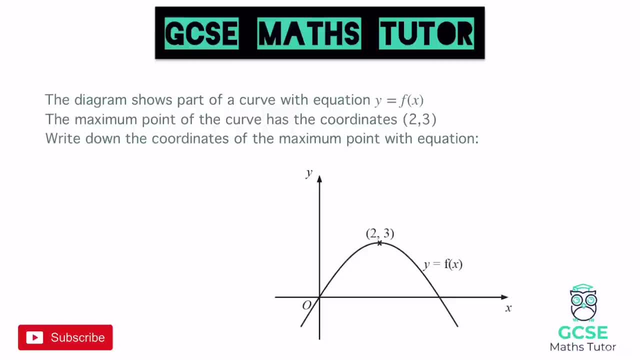 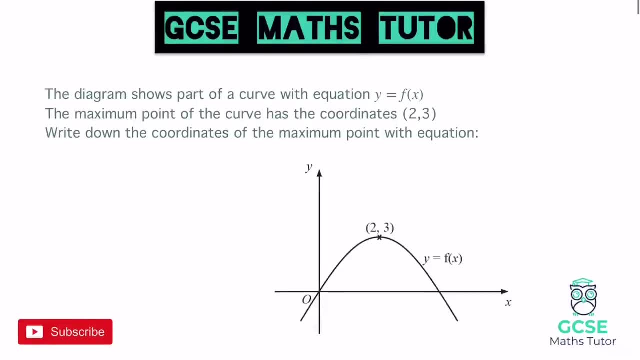 point with the equation, and we're going to discuss some of these different types of equations. okay, but this is typically how a question would be phrased. Now we can see on the diagram there, the maximum point being that this point here. if I draw on that, there we go this. 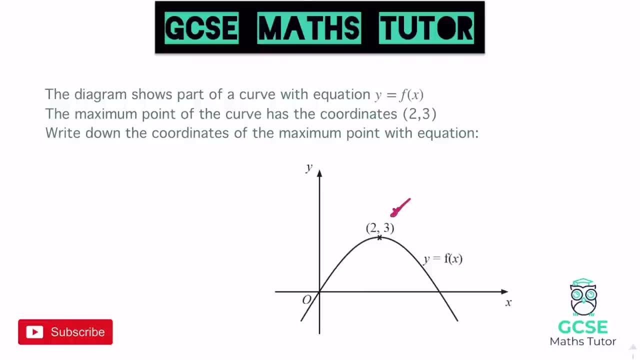 point here does actually have the maximum point 2, 3.. Okay, so I'm just going to get rid of that. but what we're going to have a look at is how we could approach different questions here. So when we change the function, we can do things either to the x coordinate. 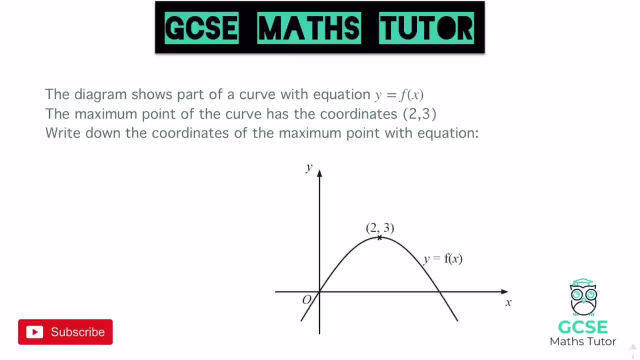 or the y coordinate or a combination of the two, and the way that we do that is by placing the numbers within this f of x, y equals f of x, and we can either place numbers or symbols next to the x or outside of the bracket, there, outside of the x. Okay, and there's a simple 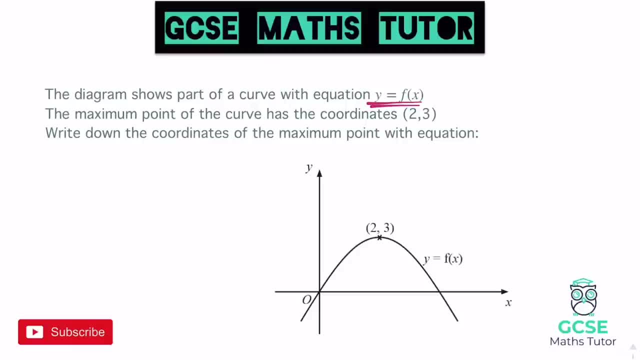 little set of instructions that you can remember for how it actually moves the coordinates. Either we're going to put things next to the x, and when I say things next to the x, I mean we can do the function of, and we could do x and we could put a plus 2 in there. next, 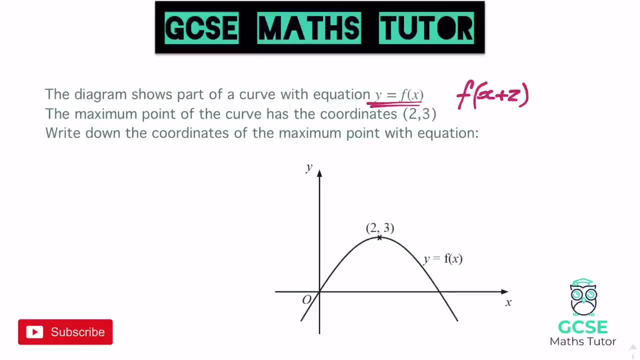 to the x. Okay, so that's one option of something we could have a look at. Hopefully, you've obviously seen these before. So either we're going to put things next to the x or we're going to put things outside of the x, which is going to affect the y coordinate. So if 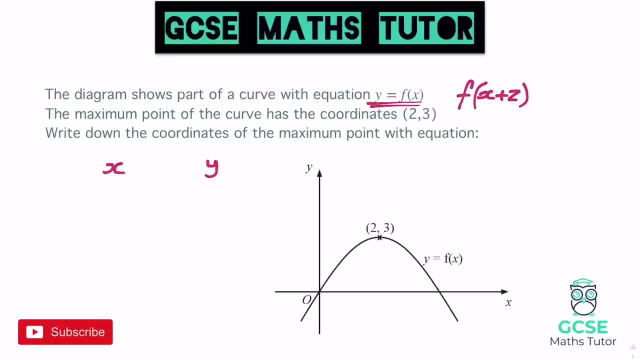 it is next to the x or inside the bracket, okay, it's going to do the opposite of what we'd expect. Okay, so it's going to do the opposite and we'll discuss that in a sec. Okay, it's going to do the opposite. And if it's outside of the brackets and it affects the y, it does. 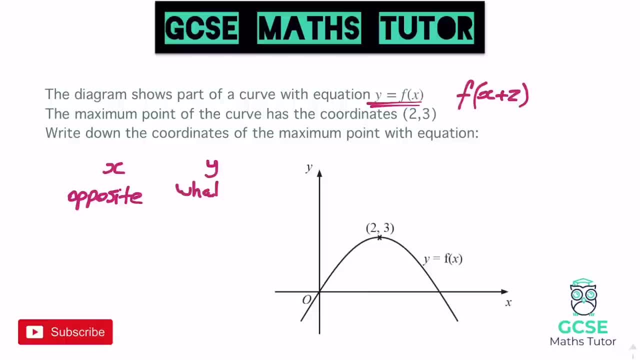 what we'd expect. Okay, what you expect. Okay. so if it affects the x, it's inside the bracket. So we'll put inside bracket, And if it affects the y, it's when it's outside the bracket. There we go. So if we can remember this little set of instructions here, it's going to help. 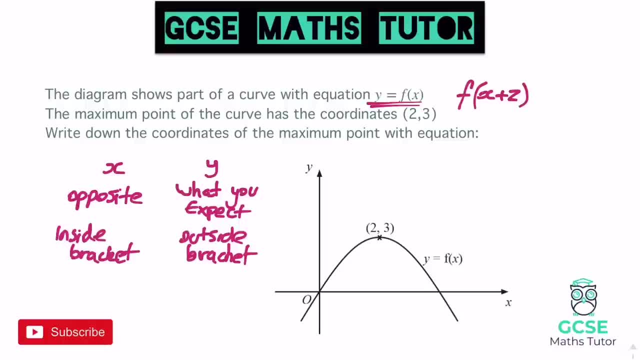 us to answer pretty much all the questions on this. So if it's next to the x, inside the bracket, it does the opposite, And if it's outside the bracket, it affects the y and does what you expect. So something like this up here, which I've drawn already: f of x plus. 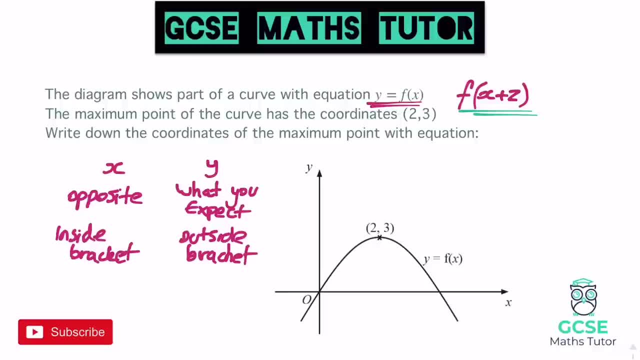 2, plus 2 there is inside the bracket. Okay, so it affects the x coordinate and it does the opposite of what we'd expect. So, rather than adding 2 to the x coordinate, we're going to subtract 2 from the x coordinate. So this one in particular, and again we're going to 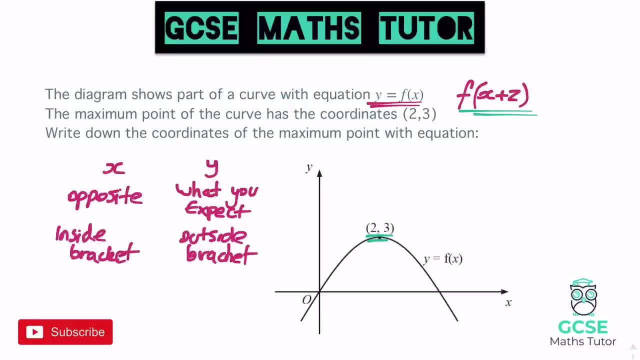 have a look at all these different types of questions. but this coordinate, here the x coordinate, there is 2.. So if I was to do this function of x plus 2 here, we would subtract 2 from the x coordinate. So 2 take away 2 would give us 0 and the y coordinate wouldn't. 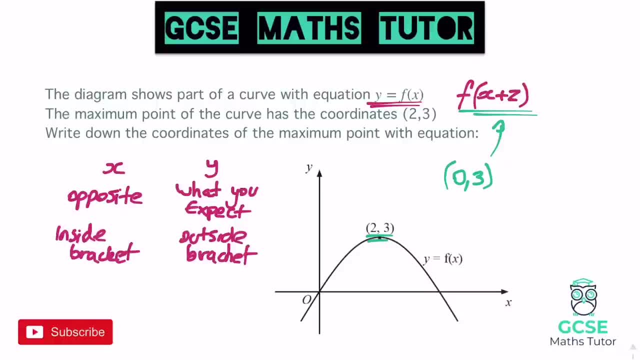 change, it would be a 3.. Okay, now, the only scenario where this doesn't actually follow- the opposite of what you'd expect scenario- is when it's a minus that we put in there- which we're going to have a look at in a sec- The minus just follows and it does what you. 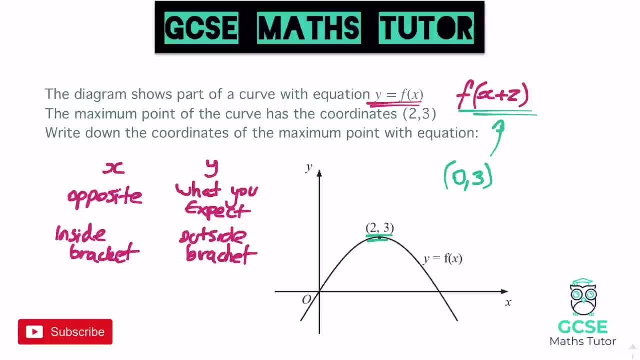 expect, no matter whether it's inside or outside the bracket, but we're going to have a look at some of these now. okay, but a simple little set of instructions there to remember and to write down. if it affects the x coordinate, it's inside the bracket and does the opposite of what you'd expect. 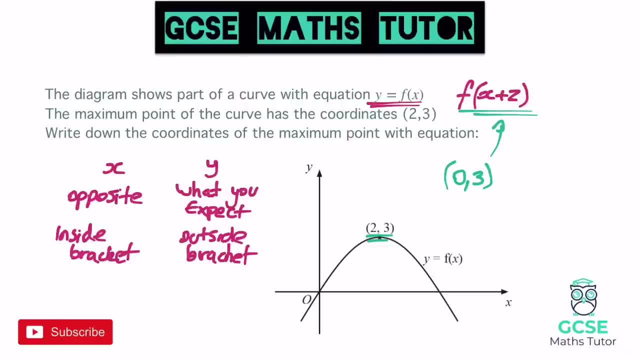 and when we're looking at the y coordinate and that's outside the bracket and it does what you'd expect. okay so, inside the bracket opposite x, outside the bracket, what you'd expect and affects y. okay so, let's have a look at some of these, okay so, same question that we were just looking at, but 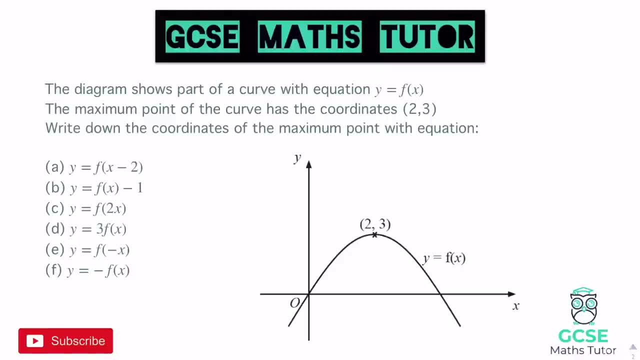 we've got some questions here that we're going to have a look at actually answering here. so it says: the diagram shows them the part of the curve of the equation. y equals f of x. and here it is in the diagram. the maximum point of the curve is 2, 3, as we've already seen, write down the coordinates of: 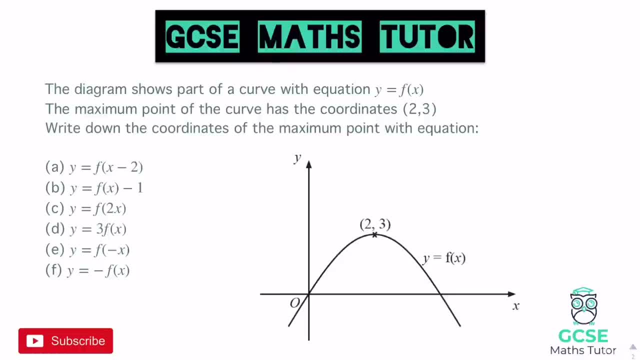 the maximum point with these different equations, and i've got quite a lot here, all the different scenarios we could actually have a look at. so for part a, there, okay, it says f of x minus 2, so that's inside the bracket, so it affects the x coordinate and it does the opposite of what we'd expect. so 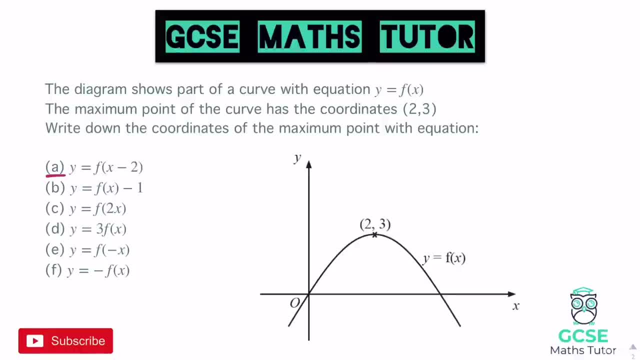 it doesn't subtract 2, it adds up to the x coordinate and it does the opposite of what we'd expect. so it adds 2. okay, so it just does the opposite. so, the x coordinate being 2 there, we would add 2 to the x. 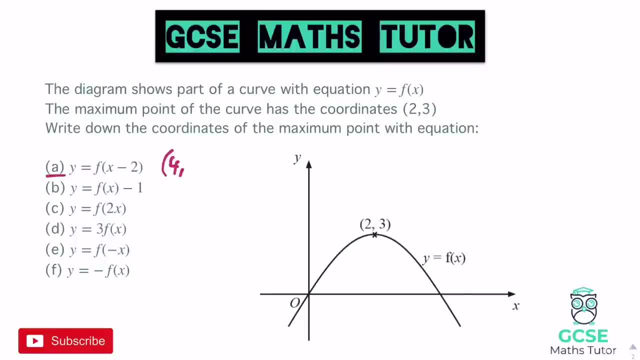 coordinate and that would make it 4, and the y coordinate is not going to change, so that would stay as 3. okay, so that's the opposite of what we'd expect, and we add 2 to the x coordinate. look at the next one. let's try to change to a different color here, right? so f of x minus 1. 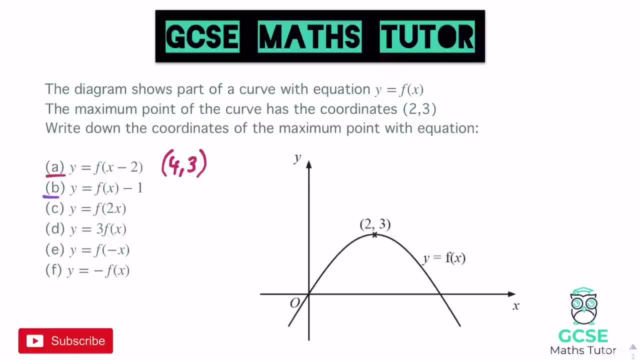 now that minus 1 is outside of the bracket. so it's outside the bracket, it affects y and it does exactly what we'd expect. so minus 1. we would expect that to subtract 1 from the y coordinate, which it does. it just changes the y intercept. actually, if you're 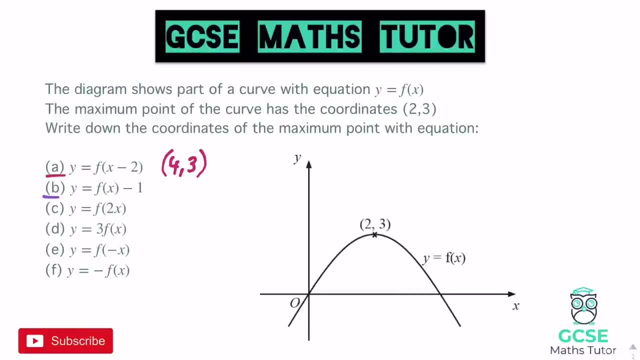 familiar with your equations of lines and your coordinates and coordinate geometry, you should hopefully know that number at the end is the y, the y intercept there. so it's taking away 1 from the y intercept, essentially just moving the graph down 1. but we'll have a look at that again a little. 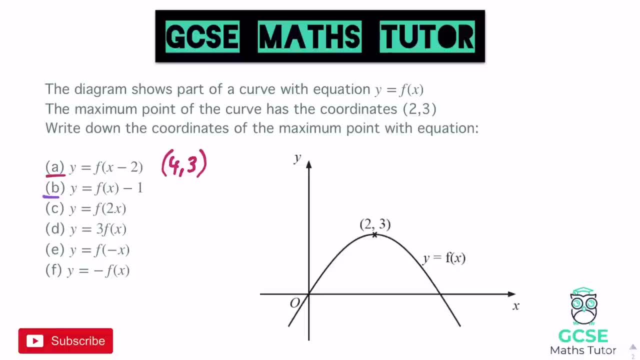 bit later, but minusing 1 from the y coordinate. the y coordinate currently is 3, so if we take 1 away from that, the x coordinate doesn't change, so 2, but the y coordinate's also going to drop down there to 2. it's going to subtract 1 from that. 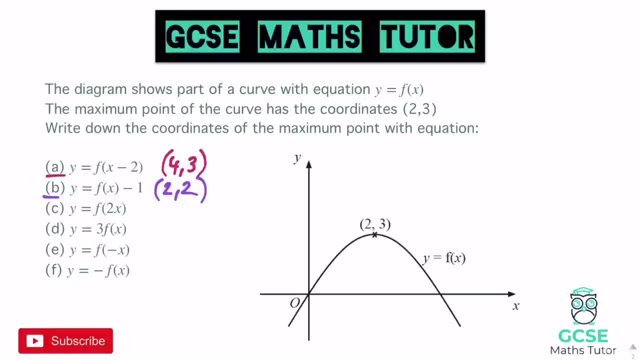 okay. so that's how we could have different scenarios there with just adding and subtracting numbers and how that affects the x and y coordinate. now we're gonna have a look at question c, part c. there so y equals f of 2x, so 2 times x. normally when you're timesing by 2, you'd expect 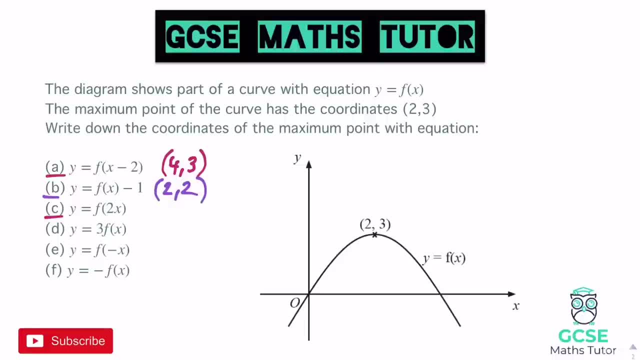 that to double something. but as it's inside the bracket affecting x, it does the opposite. so rather than multiplying by 2, it divides it by 2 or halves it there. so if we look at the x coordinate, the x coordinate is currently 2. so half of the x coordinate is 2 and half of the x coordinate is 2. 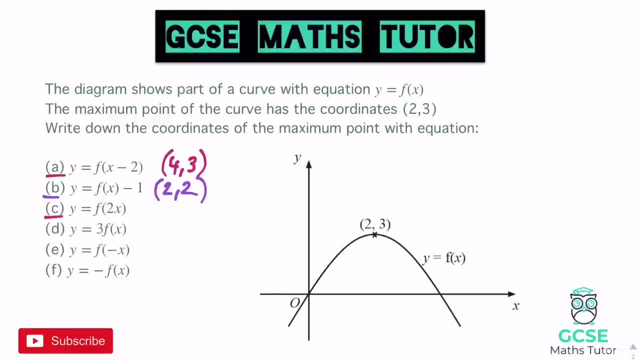 so half of that, halving it because it's inside the bracket, changing the x coordinate but does the opposite. so half of 2 is 1 and the y coordinate remains unchanged and that remains as 3. there we go. so that's that one. let's have a look at the other scenario, where it's outside the bracket. 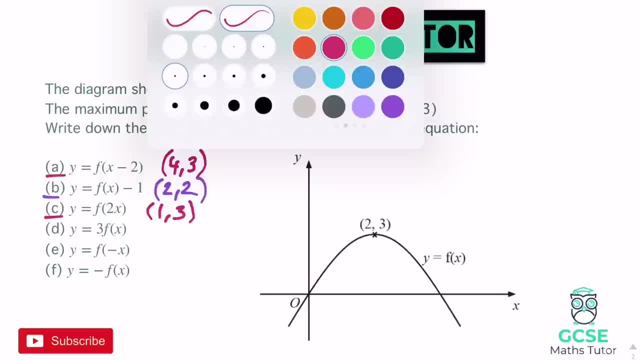 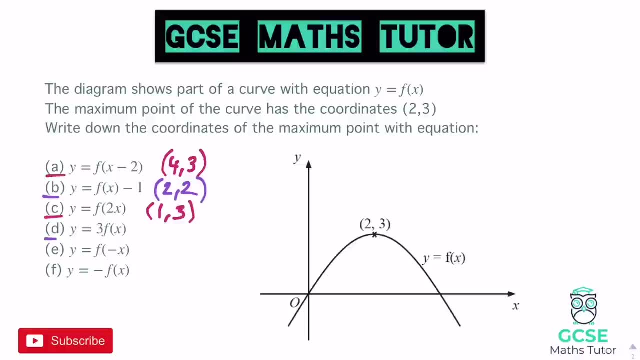 so 3 lots of f of x for part d here. let's have a look at what this does. so it's outside the bracket. it affects y. we're multiplying it by 3, so it does what we'd expect. it makes it 3 times bigger, but it affects the y coordinate this time, because it's outside the x bracket. so it's outside. 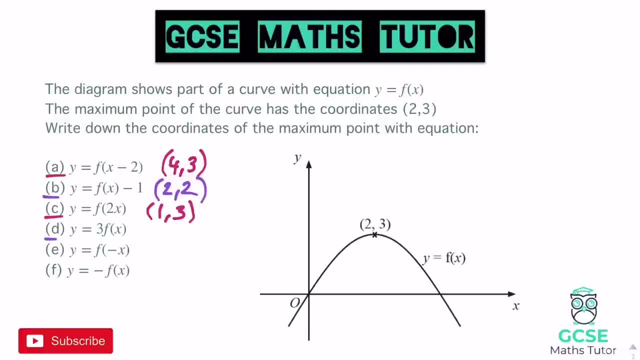 the bracket, so 3, lots of that y coordinate. the y coordinate is currently 3, so the x coordinate is unchanged and the y coordinate gets multiplied by 3 and becomes 9. right, there we go. so that is our scenarios, where we are multiplying by a number. so in terms of the x there inside the bracket, 2x. 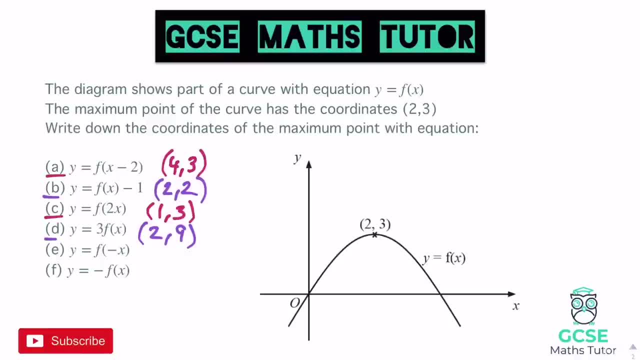 does the opposite. so divided by 2, but outside the bracket it multiplied the y coordinate by 3. okay, and onto these negative ones here, which don't really follow the same trend, but partly it does. so we'll have a look at this one here. so we've got minus x in there now. it doesn't do the opposite of what we'd expect, because the 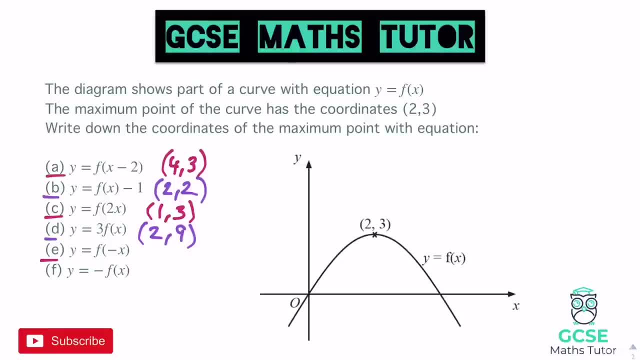 opposite of minus x would just be nothing. okay. we wouldn't actually change anything at all, it'd just be positive x. it'd be the same equation. okay, but we follow the rest of the rules for this one. it's just that it goes a little bit out the window when we look at our minuses here. so when we've 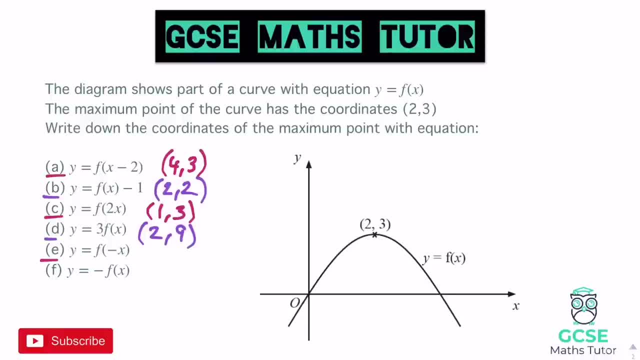 got a minus in there. all that that does is it swaps the symbol of the x coordinate. it's still affecting x, it's inside the bracket. it just doesn't do the opposite this time. okay, so it just changes the 2 as the x coordinate to minus 2. so the x coordinate's going to change. it becomes minus 2. 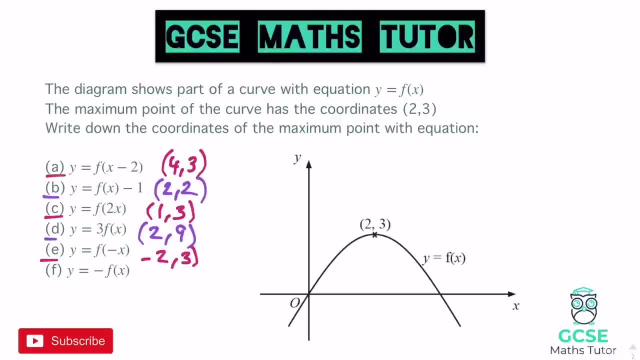 and the y coordinate remains unchanged, stays as 3. okay, so this 1 is a negative in there. that's the only scenario where it doesn't actually do the opposite or anything like that. we just have to worry about is it next to the x or is it changing the y, and it just flips the sign. so the last one, 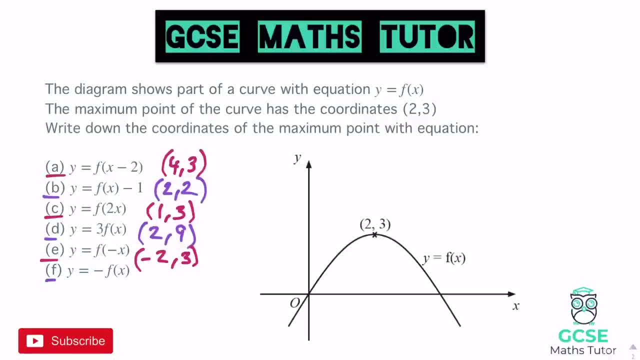 here we've got y equals minus f of x, and again the minus there is outside the bracket, so it changes the y coordinate and again it just swaps the sign. so instead of being positive 3, there is the y coordinate, it's going to be negative 3 and it just flips the sign. so the last one: here we've got y. 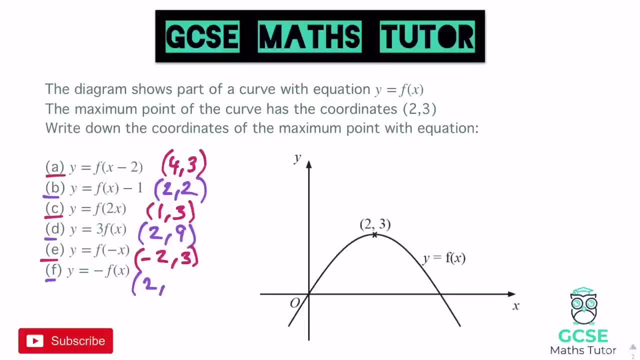 negative 3. so we have positive 2 still and negative 3. okay. so again, just following all those little rules, is it next to x, or is it next to the y or outside of the x bracket? and that tells us which coordinate of x. when it comes to adding, subtracting, multiplying, okay, we can think about. 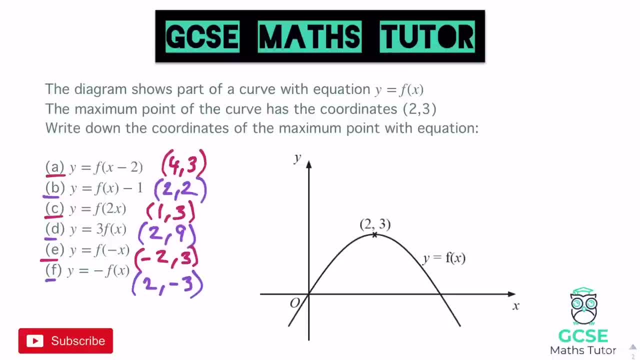 the opposite or the whether it does what we'd expect. the only scenario where it doesn't is where we've got this little minus symbol in there and that just changes the- the positive or negative symbol of the corresponding coordinate, whether it's x or y, and it just flips the sign. so the 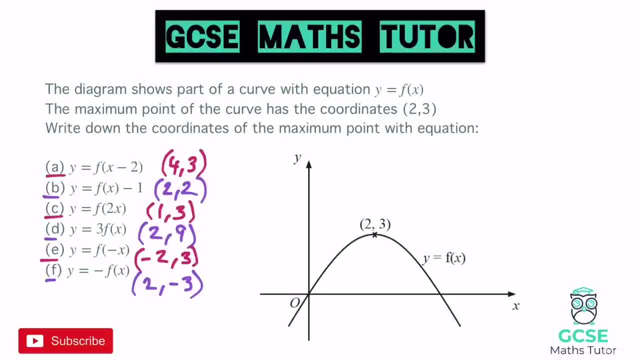 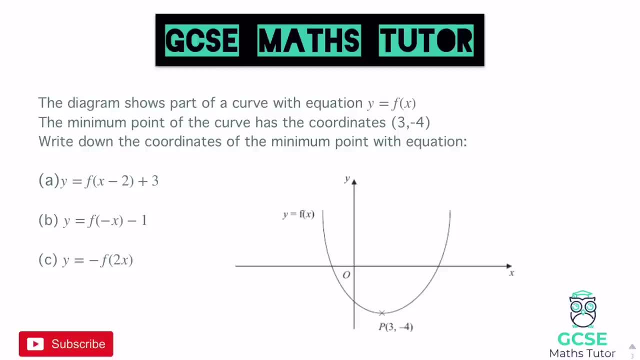 y, whether it's inside the bracket or outside the bracket. okay, let's have a look at one more. okay, so on to a different question. we've got the diagram shows part of the curve of the equation y equals f of x and it says the minimum point of the curve has the coordinates 3 minus 4. we can. 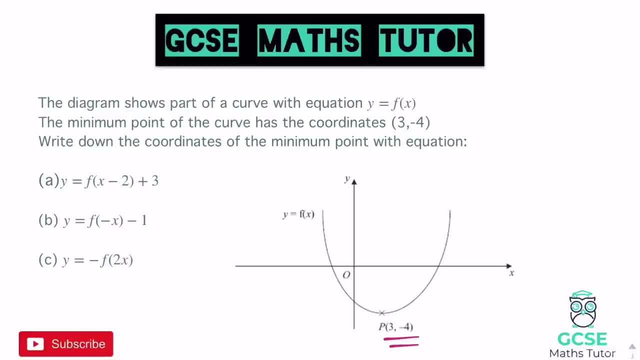 see that down here on the diagram. it then says: write down the coordinates of the minimum point with the equation. and again we've got. again we've got three equations here. now you probably notice there's a lot more going on in these. so we've got f of x minus 2 and then plus 3 at the end. 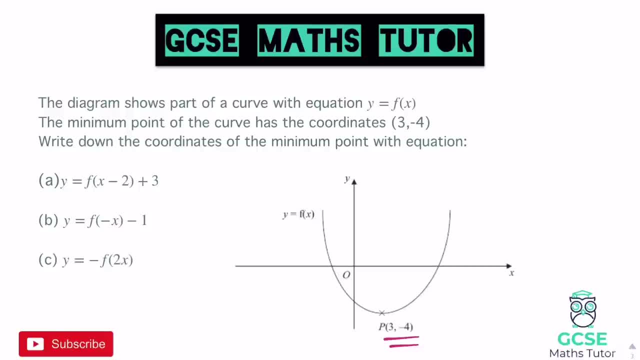 now we've got two transformations essentially, or two things happening here. we'll look at why it's happening in a second, how it moves- obviously a transformation just being how a graph moves around- so we're going to have a look at what this does. so in here we've got f of x minus 2, so we've 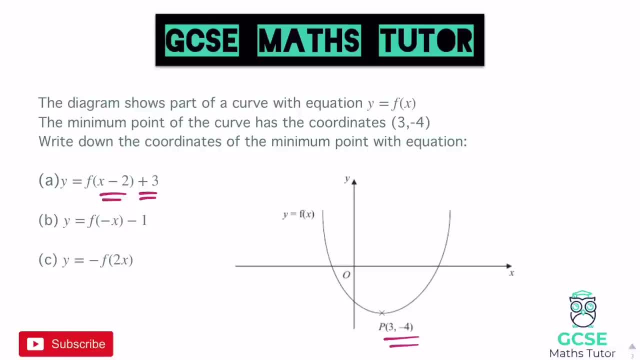 got something happening here and we've got something happening here as well. now one is inside the bracket, one's outside, so this means the x and the y coordinate is going to change. but again, we're just going to follow our little simple rules and do it step by step. so if i first start with this, 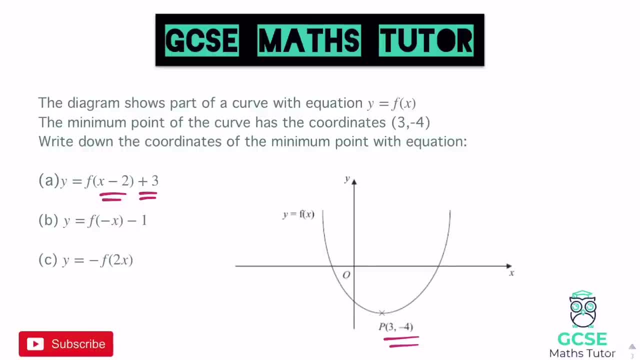 minus 2 in the bracket that affects the x coordinate. so the x coordinate is currently 3 and that does the opposite of what we'd expect. so we're not going to take away 2 from the x coordinate, we're going to add 2. so adding 2 to 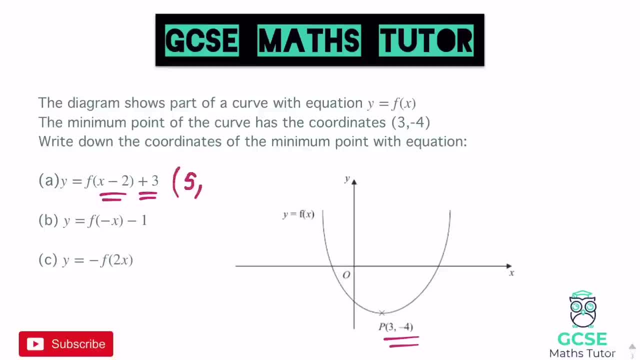 that x coordinate. 3 plus 2 gives us 5 for the first coordinate there, and that's that first bit dealt with. we've then got the plus 3 at the end and when it's outside the bracket it affects the y coordinate and it does what we'd expect. so it adds 3 to the y coordinate. so negative 4. 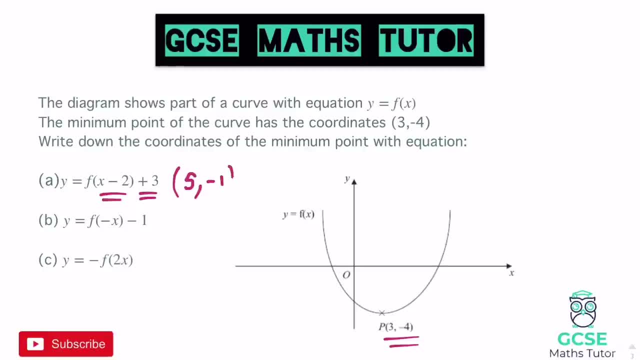 add 3 gives us negative 1, and there is our coordinate there with those two transformations. okay, so it is. if you think about what that actually does, it moves it right by two spaces, the three moves across to five and then it goes up three places as well. so if you think, 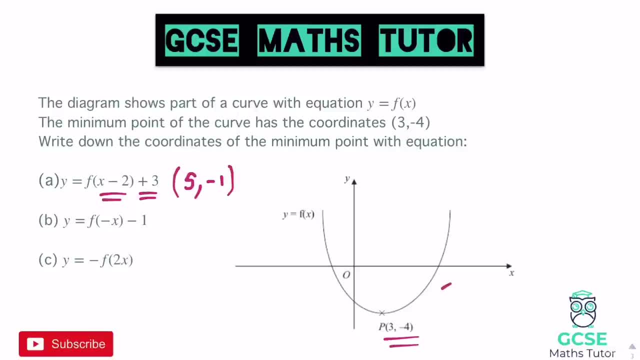 about what this is going to look like. it's going to move right and up, so it's going to be over here somewhere. that new minimum point, okay, but let's have a look, uh, what this does. if we could draw a little sketch in, okay, it would look something like this: there you go, that's what that. 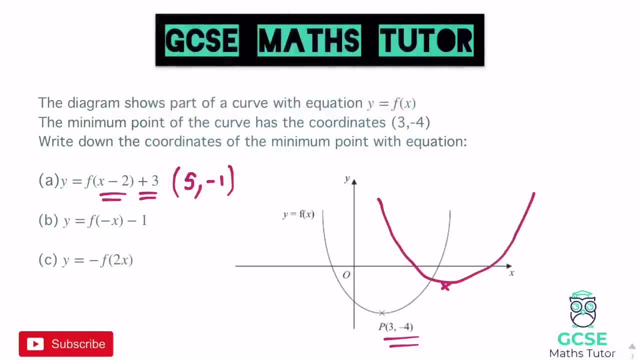 transformation would do. let's have a look at another one. so we've got the part b. it says f of minus x and then minus 1 at the end. so the minus x part that's going to swap the symbol on the x coordinate, so the current 3. 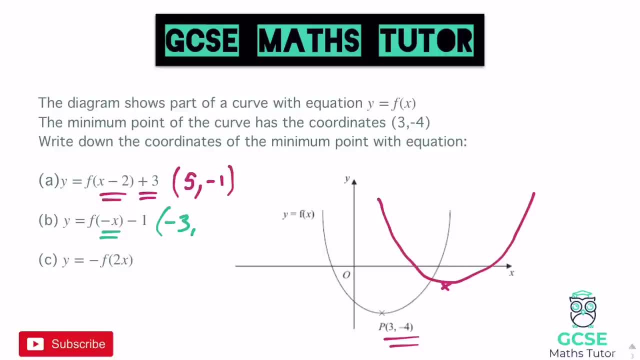 is going to become negative. 3, changing it from positive to negative again, not worrying about doing the opposite there when it's just a minus symbol. and then we've got the minus 1 at the end, which affects the y coordinate, and it does what we'd expect: it drops it by 1, so it goes from. 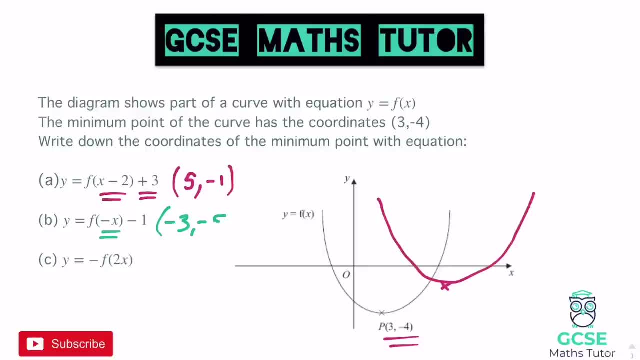 minus 4, which it currently is down to minus 5, and again, i'm doing all these questions separate from one another as if they were separate questions. so we're not going from one graph to the other, we're starting from that original graph. so i was again looking at the 3 minus 4, not the new. 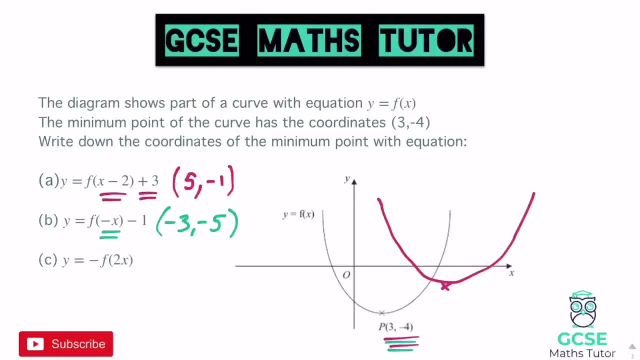 minimum point that we created on the question on part a there. so minus 3, minus 5 being our second one. and again, we'll have a look at what that actually looks like with the minus symbol there. it's a little bit more complicated for me to sketch it out on this one for you, but we will have a look at some sketching in a sec, so bear. 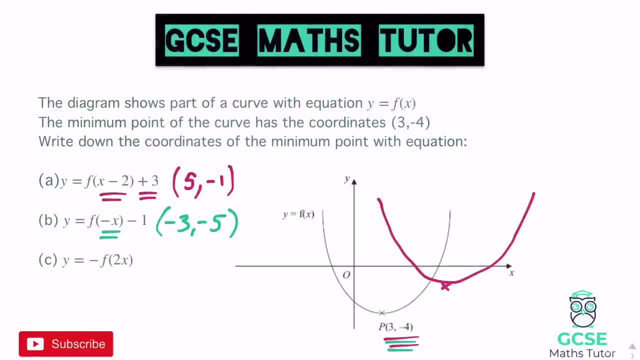 with me on that one and on to the last one. here we've got y equals minus f of 2x. okay, so this one just here. so the minus on the outside affects the y coordinate and again it flips the symbol. so if we're doing that bit first, let's have a think. 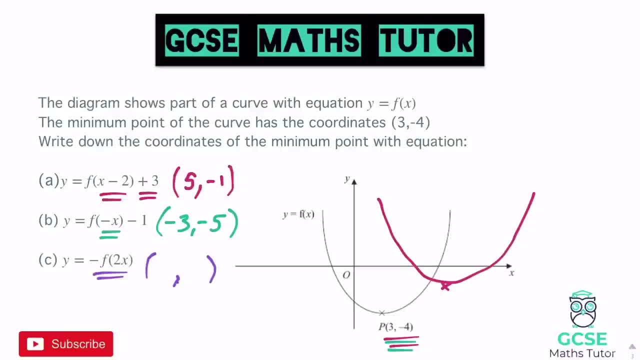 leave a little empty gap for that one there. so the y coordinate is going to change symbols, so it's going to go from minus 4 to positive 4. then, looking at the 2x, that's inside the bracket. so it is the opposite of what we'd expect. so instead of timesing the x coordinate by 2, it's 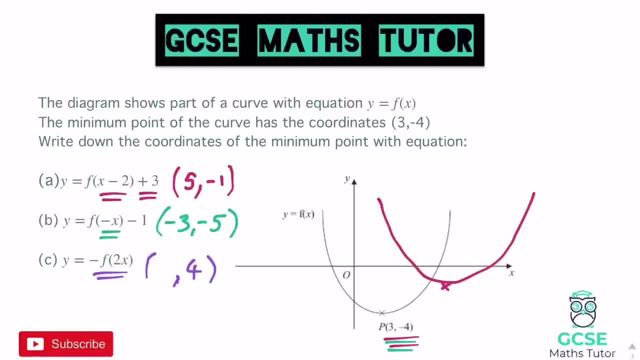 going to divide it by 2, and the current x coordinate is 3. so dividing that by 2 is not going to give us a whole number there, it's going to give us 1.5. there we go, we can have decimal coordinates as well. that's absolutely fine. it's fine. it's just halfway between 1 and 2, isn't it? 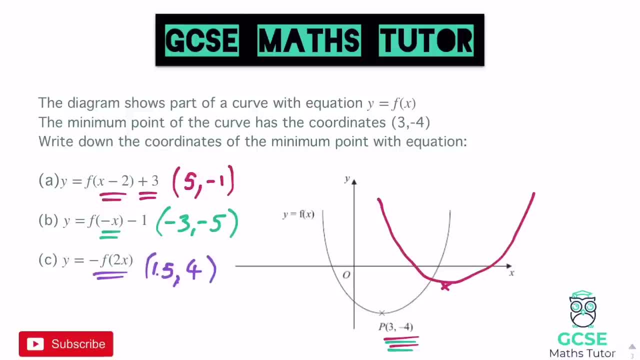 so 1.5 is going to give us 1.5, and then we're going to divide it by 2, and then we're going to have 1.5 being our x coordinate. okay, so that is how our transformations are going to work, so just. 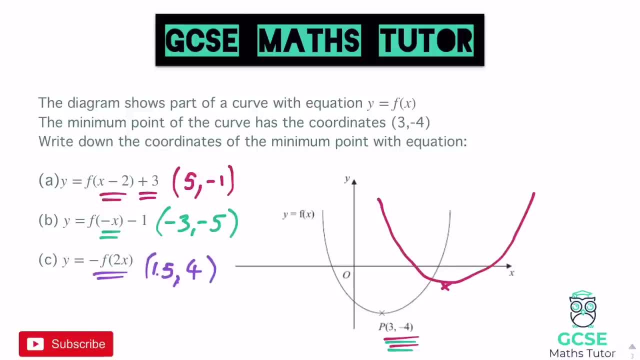 remember that little table. if it's inside the bracket, it affects x and does the opposite of what you'd expect, and if it's outside the bracket, it affects the y coordinate and it does, logically, what you'd expect there. the only scenario where it doesn't is obviously with the minus symbol. 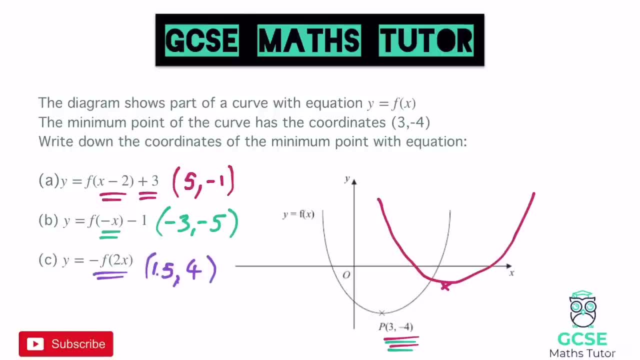 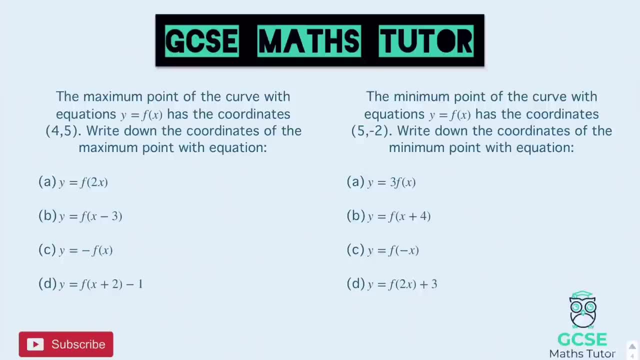 and again, that's only when it's inside the bracket. it just does what you'd expect there. it just doesn't do the opposite. okay, so here's a couple for you to have a go at. okay, so, quite a few questions on this. you've got two questions, one on the left, one on the right, and four parts on each. 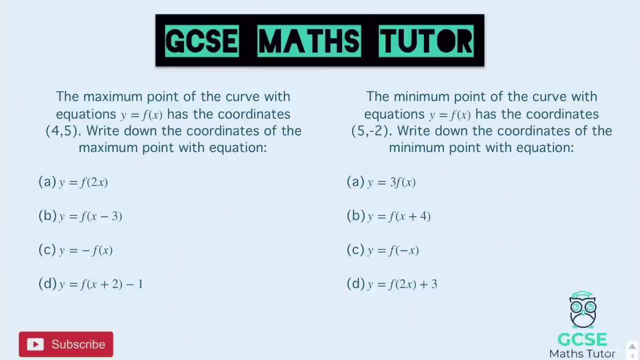 one. you've got the minimum points on each one. you've got the maximum point on the first one. you've got a minimum point on the first one. they're the coordinates that you need to change, so have a read through. pause the video there and we'll go over the answers in a sec. 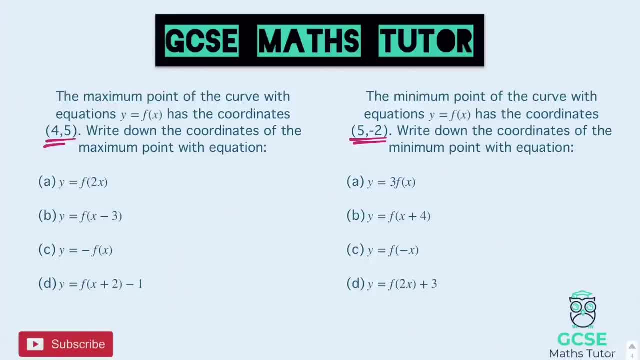 okay, so looking at the first one, so part a for this one divides the x coordinate by two, so we would have 2, 5, the opposite of what you'd expect there. changing the x coordinate onto the next one, changing the x coordinate, and then we've got the minimum points on the first one. so we've got the 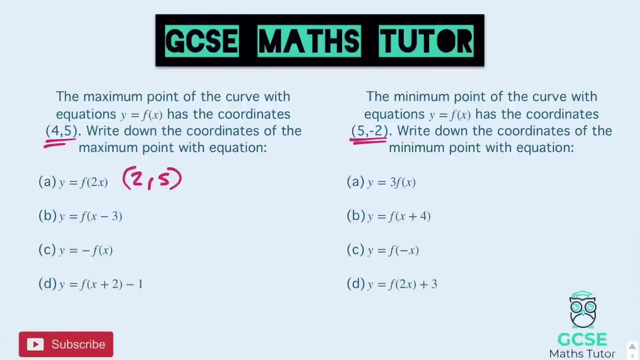 x coordinate again, but it does the opposite of what you'd expect. so adding 3, 4, add 3 is 7 and the y coordinate again is unchanged. so 7- 5 onto this third one negative on the outside, so it changes the y, so we're not changing the x, so that stays as a 4 and y becomes negative, so it becomes minus 5. 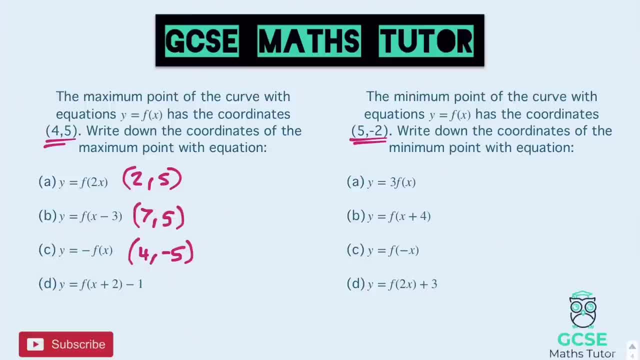 and now onto the last one. we've got two transformations to do. we've got to subtract 2 from the x coordinate- the opposite there inside the bracket, so 2, and we've got to take away 1 right onto the second one here, so we've got 5 minus 2 as our coordinate, so 3 on the outside of. 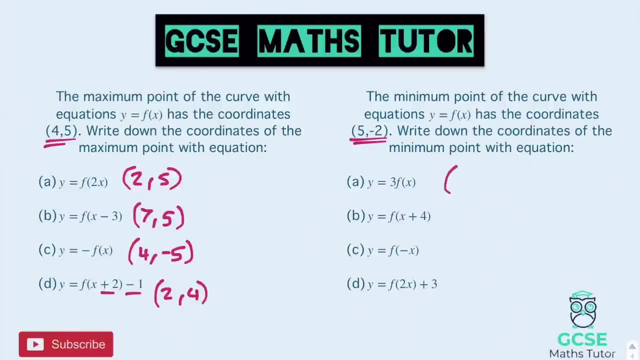 the bracket for part a multiplies the y coordinate by 3, so it becomes 5 minus 6. part b inside the bracket, subtracting 4 from x, so we have 1 minus 2 onto part c minus x. so that's going to change. 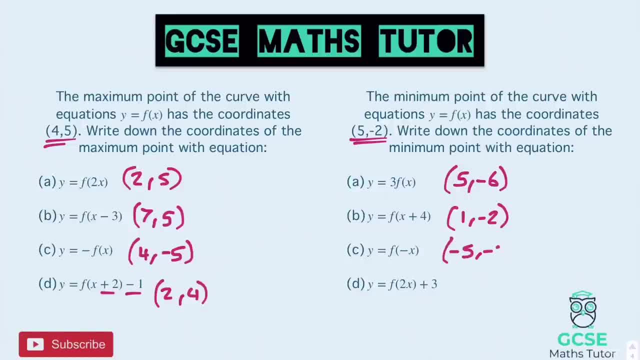 the x coordinate symbol. so minus 5, minus 2 and onto the last one. here two transformations we've got: dividing the x coordinate by 2 and adding 3 to the y coordinate, so the x coordinate is 5. divide that by 2 is 2.5. and then adding 3 to the y coordinate sends it from minus 2 up to. 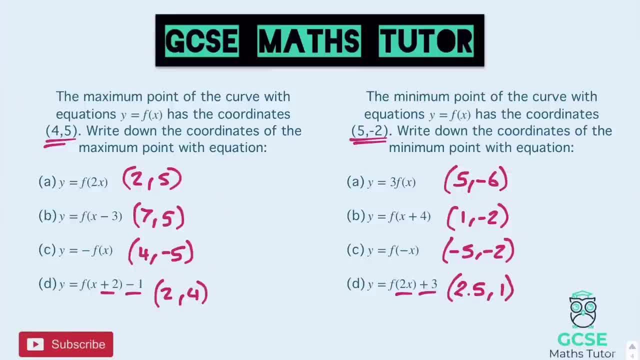 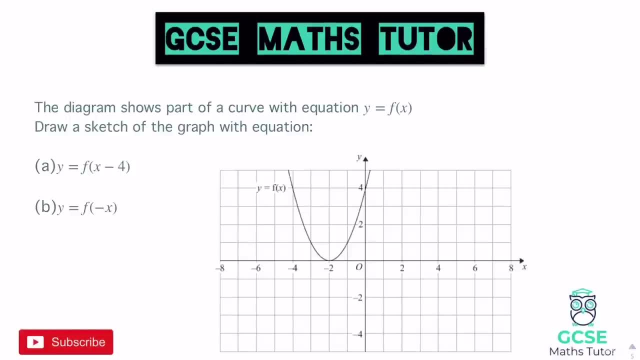 positive 1, so it's 2.51. right, let's have a look at sketching some of these. okay, so it says the diagram shows part of a curve of the equation y equals f of x. draw a sketch of the graph with these two equations. i'm going to do two on one graph just to save a bit of time here. so part a: 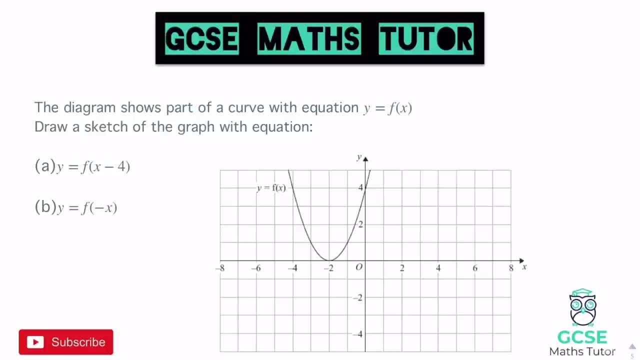 says to draw y equals f of x minus 4. now we know that x minus 4 here is going to plus 4 toward the x coordinates. so add 4 to x. okay, now what we've got to do is make sure that we find any whole number coordinates on this. 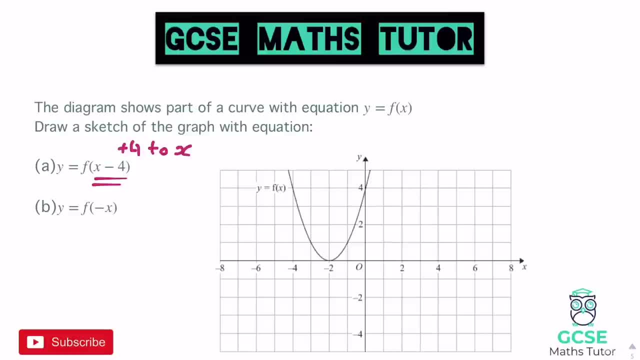 graph and they're the key ones. so i can see quite a few and i'm going to highlight them here. so we've got one here, we've got one here and we've got a few down the bottom here that go through actual whole number coordinates. so they are the coordinates that i need, to make sure i 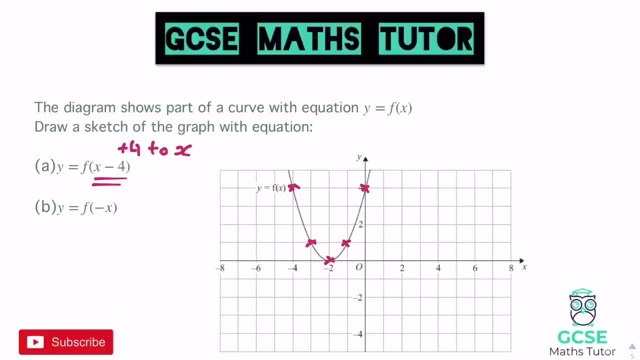 move perfectly when i'm drawing my little sketch the rest and we can just do it as accurately as we can. so if we're going to add 4 to the x coordinate, well, let's look at this one here to start with that coordinate, there currently is 0, 4, so when 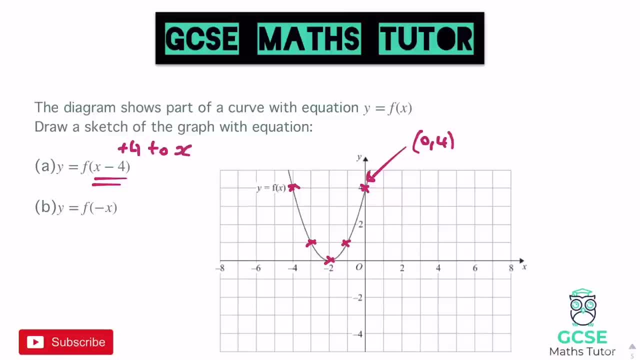 i add 4 to the x coordinate, that is going to become 4, 4. okay, adding 4 to the 0, so 4, 4 is the coordinate here and you can see there. that's moved it right. four spaces and that's what that could. 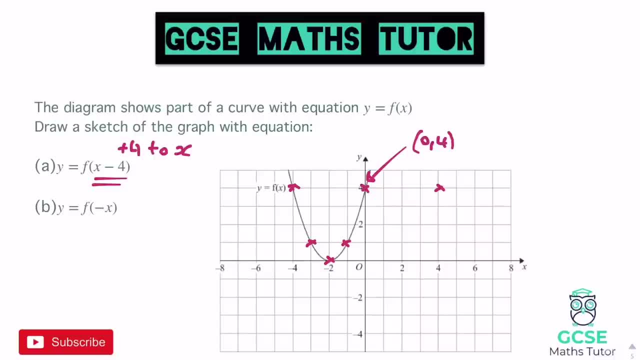 actually that transformation there actually does okay. so when we actually add 4 to the x coordinates, we're going to get 0, 4 and therefore it's going to be translated okay to the right. okay, so we're translating it 4 to the right. now, looking at the other one, um, this one here, if i move that 4, that's. 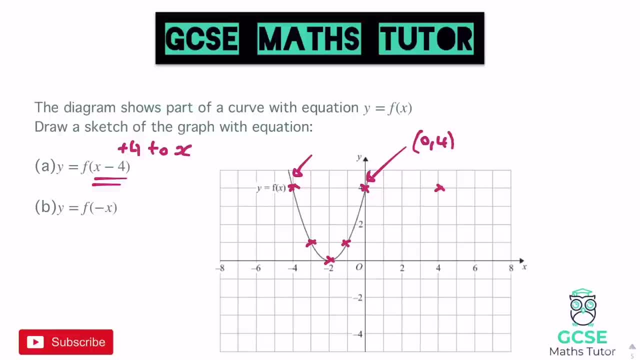 going to land on top of that 0, 4 coordinate, so i can't draw over the top of that. that's where that's going to move the one down the bottom here, this minus 2, that if we move that right 4 that's going to go to here and then moving the others right 4 is going to place them there and 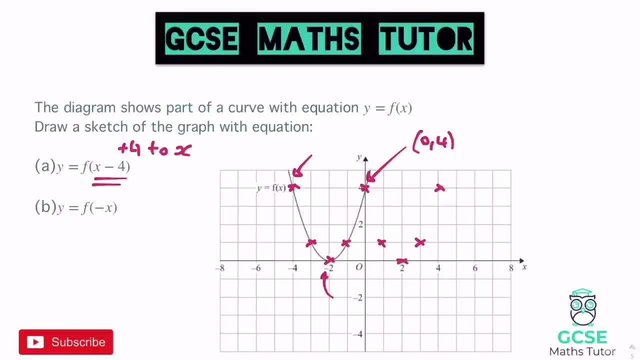 there. there we go, and that is how they would move now if i just move that right 4 and i move that right 4, we're going to get rid of some of these bits here because we're going to do another one in a sec. let's get rid of all of them and let's just sketch that in, and you've got to just do this nice. 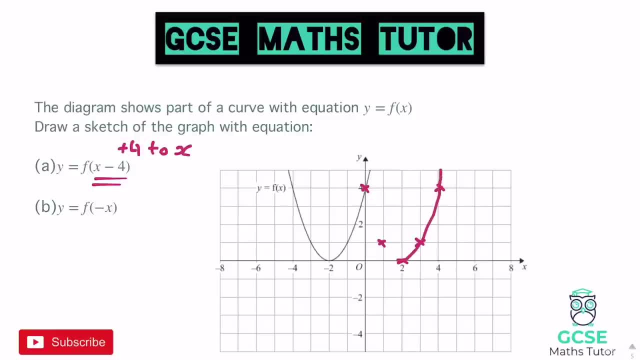 and neat. okay, as best you can, drawing a nice smooth curve, making it look as best as you can, like the one on the graph there. there we go. it's not perfect with my lines there, but just moving it right. 4 and showing that it goes through those whole number coordinates. and let's have a look at 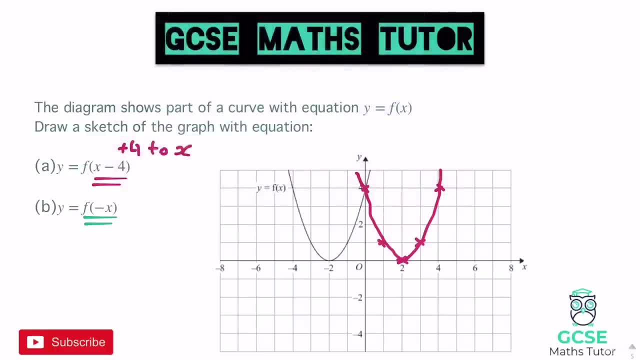 part b: here we've got y equals f of minus x. now, minus x, we know, changes the symbol on the x coordinates. so again, if we pick a coordinate and let's pick this one to start with, okay, so this one here, let's label this over here. that coordinate there is minus 2, 0, okay. so if we swap the symbol, 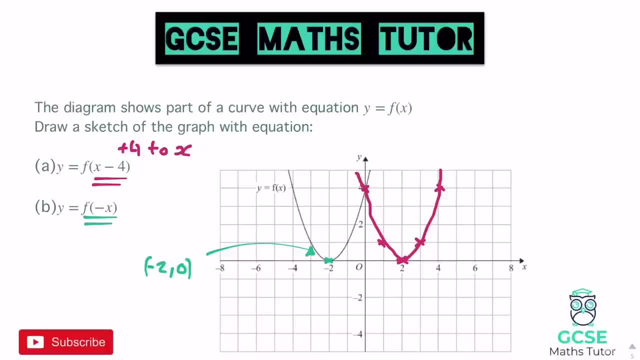 on the x coordinate there. that's going to become positive 2 0. okay, so positive 2 0 again. let's get rid of this first graph. positive 2 0 is here. there we go. let's have a look at another one. um, let's pick this coordinate here. 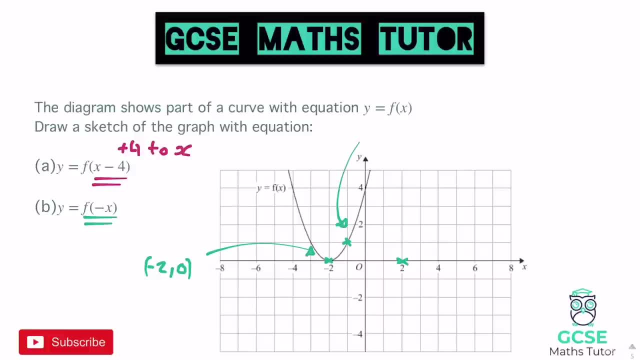 there we go, so that coordinate there is minus 1, 0 and if we change the symbol in front of the x coordinate, that becomes positive 1 0. so positive 1 0 is there. and let's have a look at one more down here on the bottom we might be able to figure out where the rest are going to go afterwards. 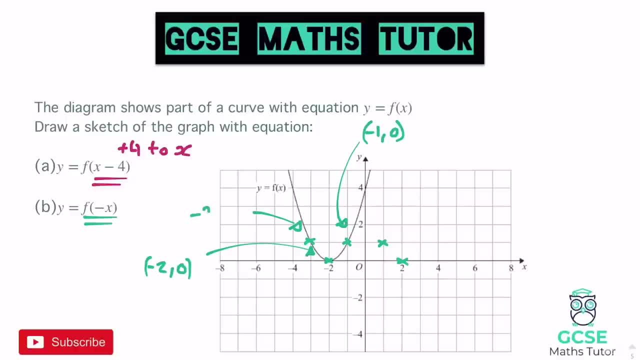 this one here is minus 3: 0 and again swapping the x coordinate, now that becomes positive 3, 0, which is just here. so hopefully you can see it. actually, this curve is going to end up in exactly the same place as the last one, but what's actually happening here? let's have a look. let's just get rid. 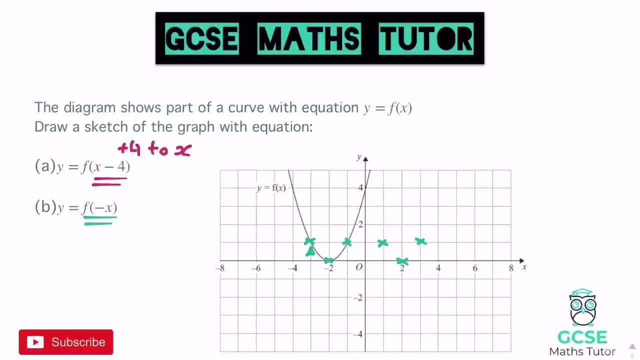 of all this- so we can see it a bit better- is something slightly different to the last one, because that last one was a transformation. it was actually moving right for, whereas if you have a look at- and i'll try and do them in different color- here this coordinate, here the purple one. 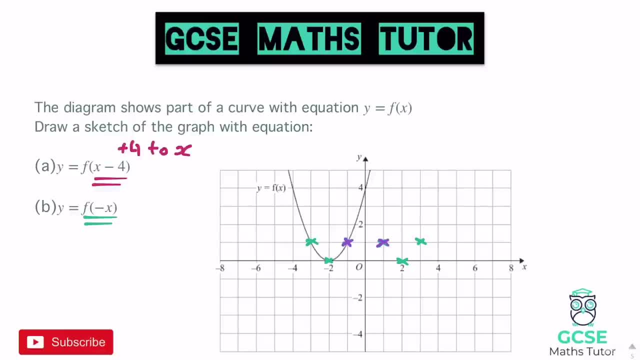 moved to this coordinate here, so actually it's not being moved in the same way, because, as well as this coordinate here has moved to this coordinate here, what this is actually doing is reflecting the shape in the y-axis, okay, and you might actually be able to see that this coordinate. 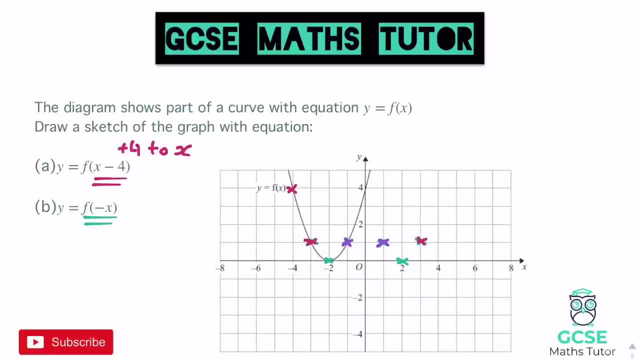 here as well, would move to. let's make sure i do this carefully now. i'm not writing down the coordinates. it would move to there and the coordinate which is here on the axes is not going to move anywhere. it's going to stay where it is. so, actually, what's happened is the curve has. 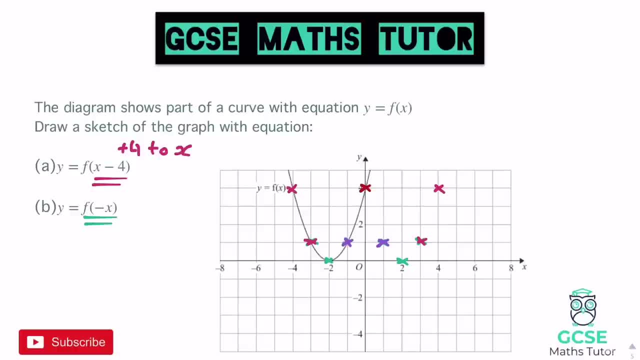 been reflected. but actually all you've got to do is reflect those or change the symbol in front of those x coordinates and again just sketching it in nice and neat. so it's quite unique there because, oh, there we go. not very good there, make sure you do go through. 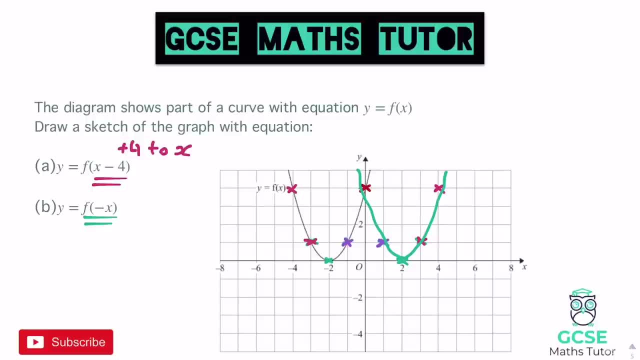 the coordinate points. but although there were two different um transformations there, two different changes in the function, the graph did end up in the same place, but there were different transformations. one's a reflection and one was a translation. okay, but as it turned out, they ended up in the same place for that one. but let's have a look at another one. okay, so we've got a different. 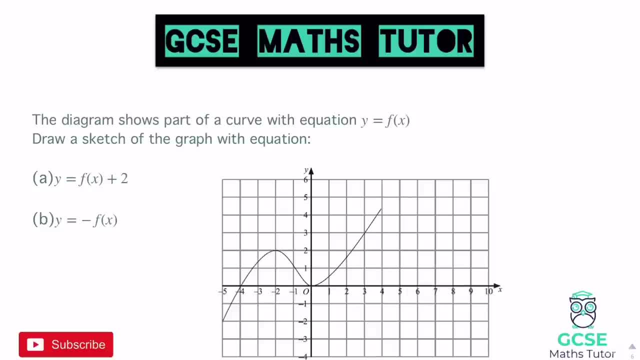 curve. here we've got the diagram shows part of a curve with equation y equals f of x. draw a sketch. so again, we've just got some slightly different ones here we've got the first one being f of x, add two. now we know that that adds two. so plus two to y, there we go. so again, all we need to do is find. 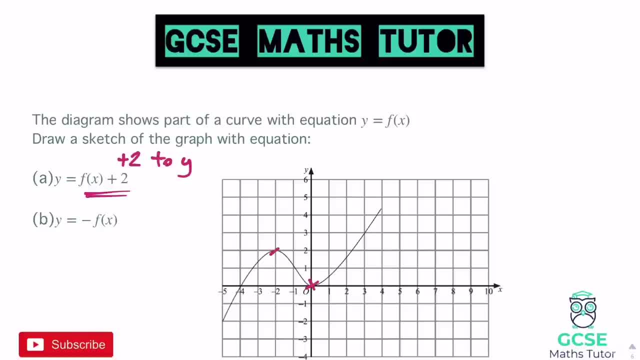 these whole number coordinates. we've got one here, we've got one here, another one here, another one here. i've got quite a few on this one and another one there. so if i want to add two to all the y coordinates, let's start with this one, the y coordinate. here is three: the um, the coordinate. 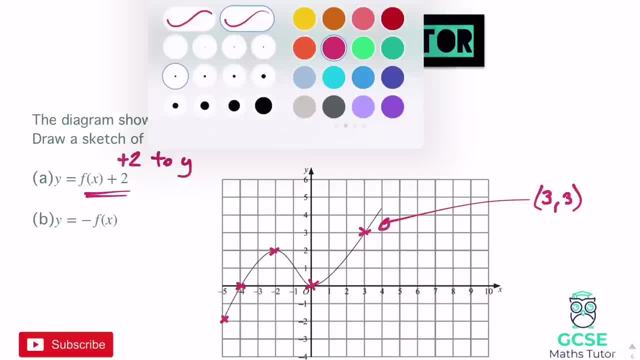 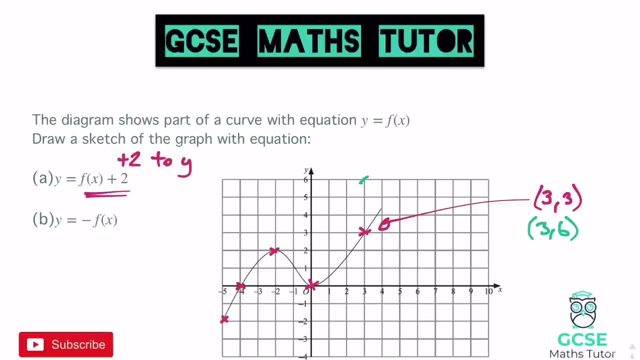 is three, three. so once we add three to the y coordinate that's going to become three, six. okay, so three, six is here. so essentially it's just moving up three, okay, so we can just do that. quite nice and easily. now for the rest of them, we can just move them all up three. so going from right. 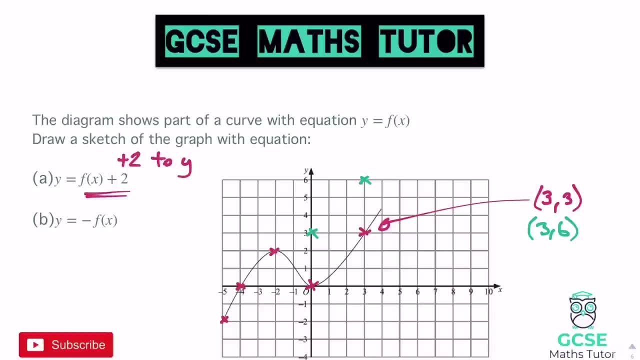 to left. if i move this one up three, it goes to here. if i move the next one up three, it goes to here, the next one up three goes to there and this final one up three goes to here and this final one goes to here. and again, just drawing that in as best as you can through all those whole number. 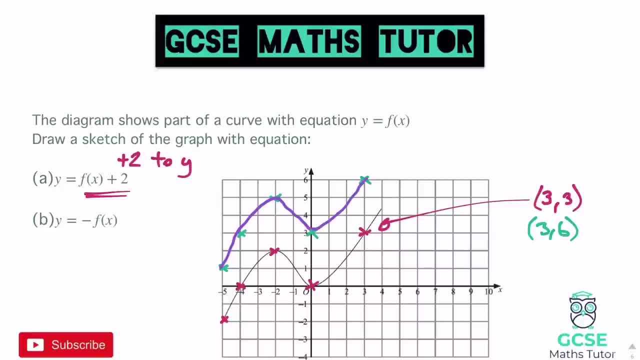 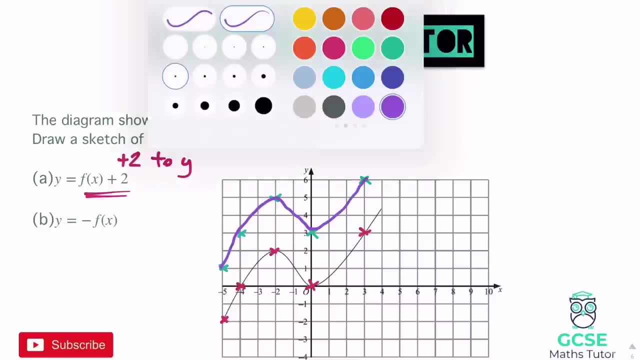 coordinates, replicating what the graph below looks like. and there it is moving it up three. okay, so nice and simple there. once you've got your one coordinate done, you can tend to get all the rest done quite nice and easily. let's have a look at part b. it says y equals minus f of x. so it's. 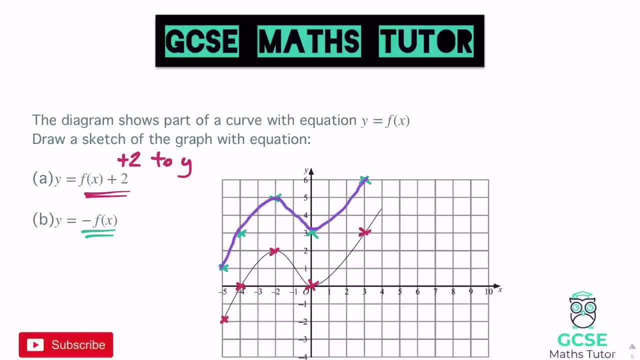 outside the bracket. it's going to change the y coordinates. so, similar to what we did in the last one, but the y coordinates are going to change. so again, if i have a look at this one just here, it's going to change the y coordinate to a minus, so it's going to become three minus three and three. 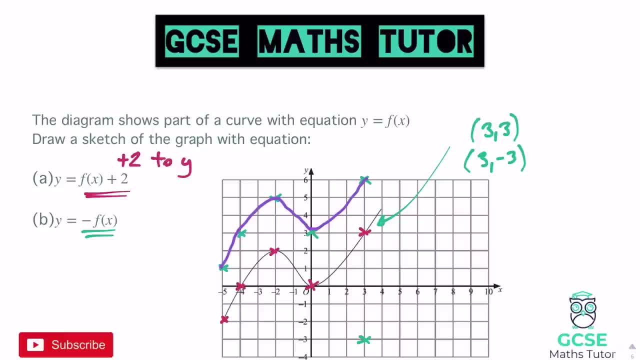 minus three is down here, okay. so, as you can probably see actually what's going to happen here, it's going to reflect not in the y-axis this time, but in the x-axis, and this is what this is going to do. so if you change all the y coordinates and flip the signs, actually it's going to do a. 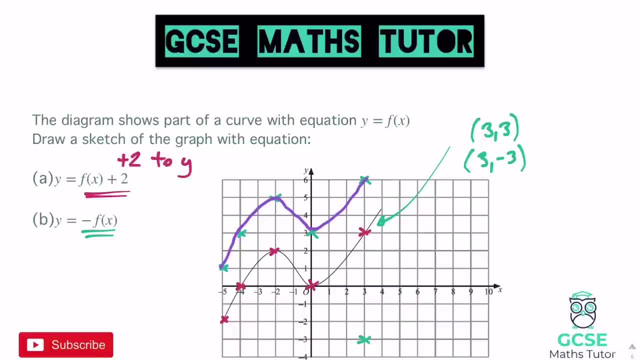 reflection in the y and the x-axis. so if you have a look at this next coordinate, that's on zero zero. that's not going to change. zero zero is still going to be zero zero, so that stays where it is. moving on to this coordinate, this one's minus two two, so that's going to become minus two, minus two. 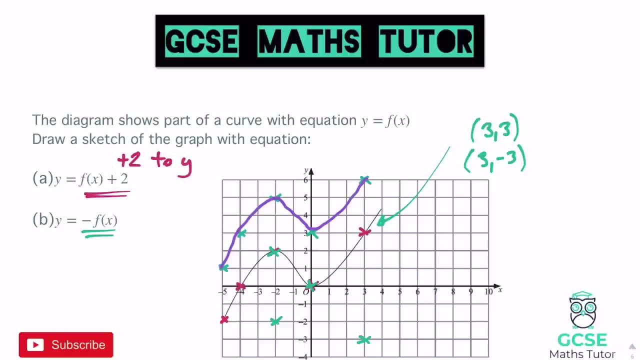 changing the y coordinate there, and the next one is on the x-axis, so that's minus four zero. that's going to stay as minus four zero. and the last one here is minus five minus two, and that's going to become minus five plus two. that's going to go there, right? so you've got to be a little bit. 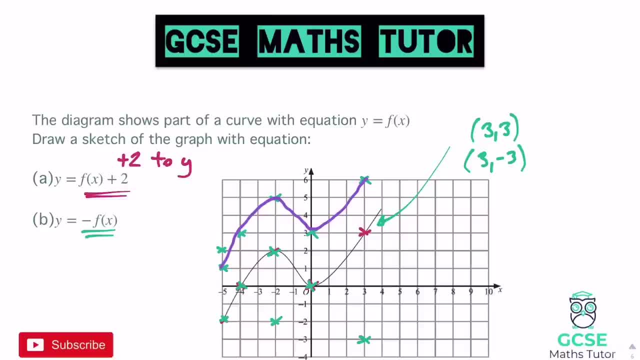 careful now when you're drawing these because it's a little bit more complicated to draw. but if i connect them all up, you can see it goes up to here, down to here and up to there. okay, so try and get rid of that one on top. there we go, let's get rid of that one. 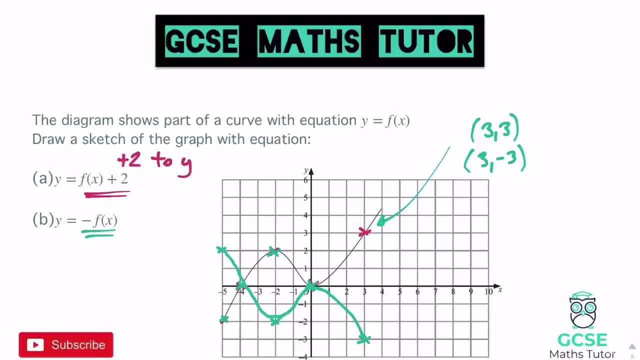 so in this case here, that has actually done a reflection in the x-axis, and you've got to be very careful to draw that in as best as you can. okay, so you've got a few different ones, you've got the movements or the translations, left and right and up and down, but then you've also got 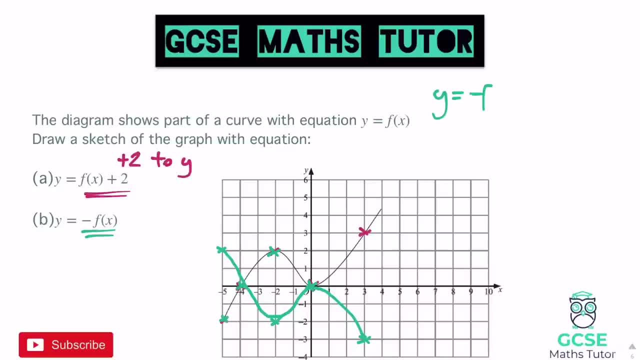 these ones here. so y equals minus f of x does a what we've done here, which is a reflection in the x-axis. and you also have the one that we looked at on the last question, which is y equals f of minus x, which does the opposite. there you've got a reflection. 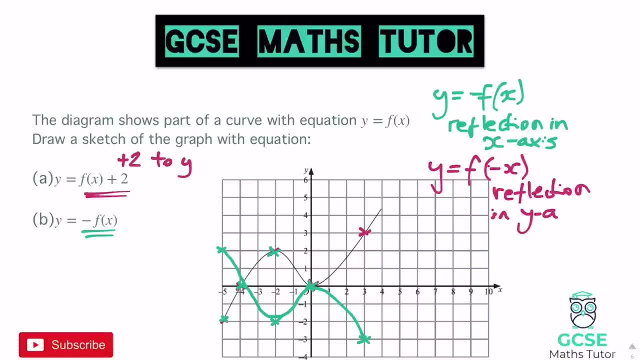 in the y-axis? okay, but each time that you do these, really as you know how to move the coordinates, now all you've got to do is pick those whole number coordinates and just change them as the function transformation actually says to do there. okay, so if you need to add two to y or take away two from x, or change the symbol for x, 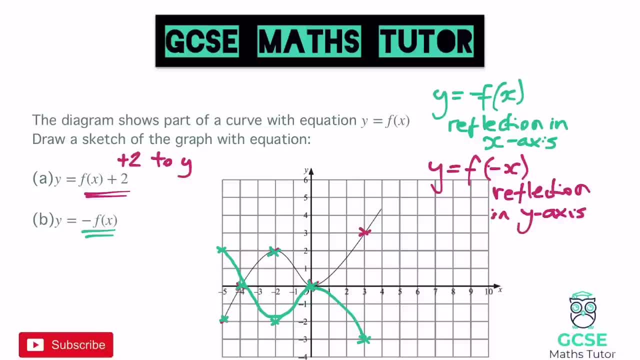 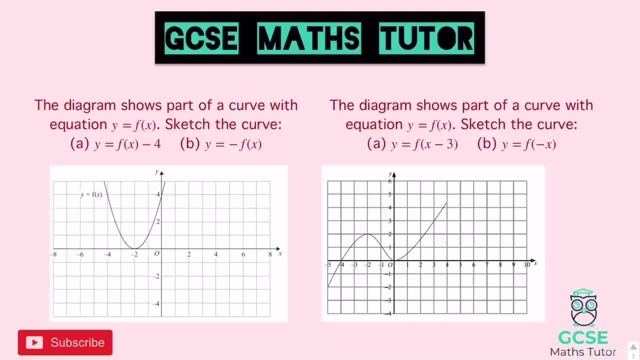 and y, just do that and draw them in nice and carefully and connect them up and take your time with it. okay, so here's two for you to have a go at. okay, so you've got two questions here. obviously don't expect you to actually draw these, but have a think about where they would move and how they. 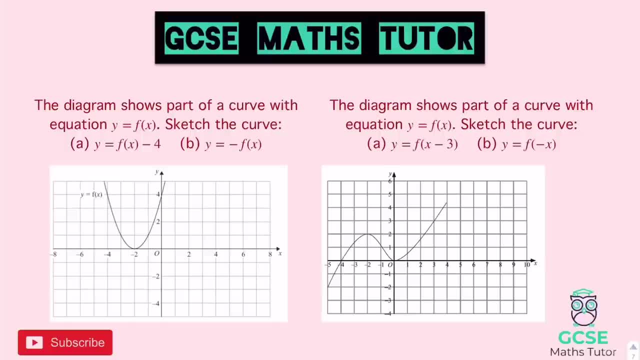 would look. you can always draw a little sketch of them if you want. it's not too. it'll be too difficult just to do a little sketch. you won't be able to do the coordinates perfectly unless you've got some graph paper, but you could actually have a go at just thinking about what they're going to. 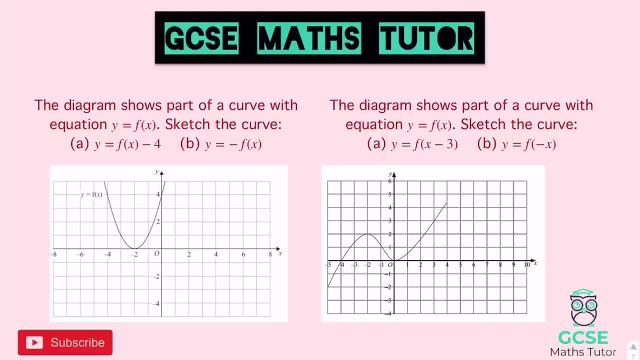 look like on the screen. okay, so for each question there are two parts, part a and b. so have a go think about where they'd go pause the video there. we'll give the answer in a sec, okay, so this first one. so if we have a look at this one to start with, we've got a minus 4 on the outside, which 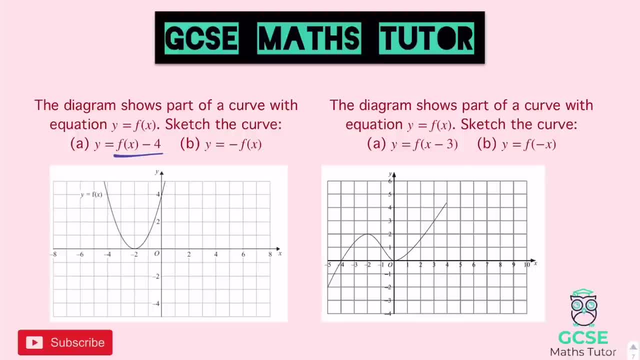 changes all the y coordinates. so essentially it's going to move down 4. so if we start with this bottom minimum point here, that's going to go down 4, down to minus 4, and then all the rest of these whole number coordinates here which I'll 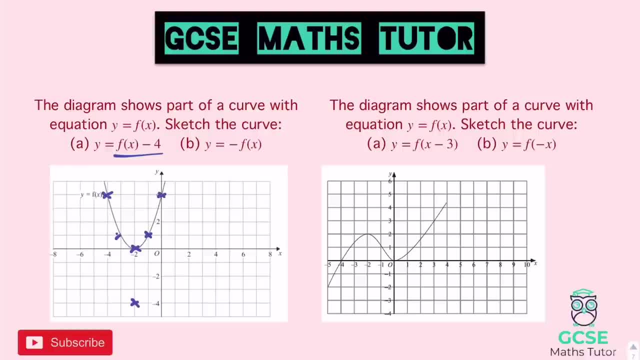 highlight, are all going to go down 4.. And if I just move them all down 4, that's going to be here and here, and then those upper ones are going to go down 4, down to here and here And again. 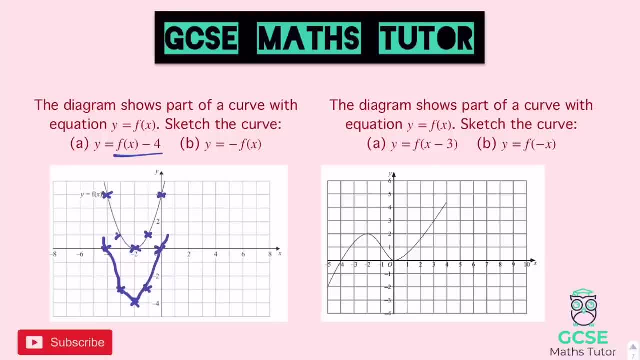 I just need to try and draw a little sketch of the graph that I can see. and there we go, as best as you can, Right on to the next one. We've got minus f of x, so that's outside the bracket again. so it's going to affect the y coordinates and it's going to flip the signs. 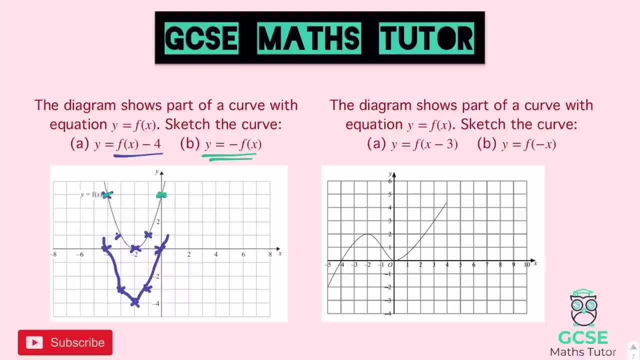 on them. So these top ones up here which have y coordinates of 4, are going to go down to y coordinates of minus 4, negative 4.. There we go. The 1 on the axes here isn't going to change. 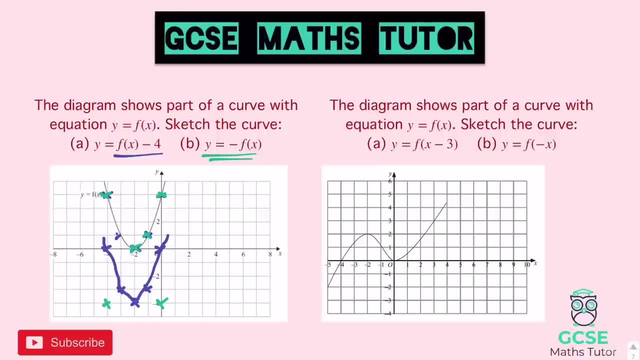 because the y coordinate is 0, but these two are going to change here. These positive 1 y coordinates are going to go down to negative 1.. There we go And, as you can see, that's done. our reflection there in the x axes. Okay, so just making sure you go through all those whole number. 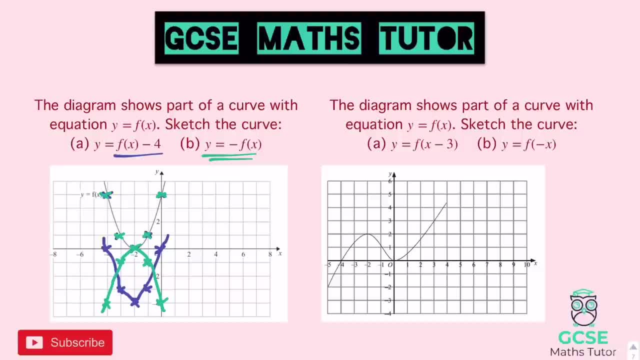 coordinates. Now, you normally wouldn't have two on top of each other like that, but so we've got a two on each one. So let's have a look at the next one. We've got y equals f of x minus 3, so that's. 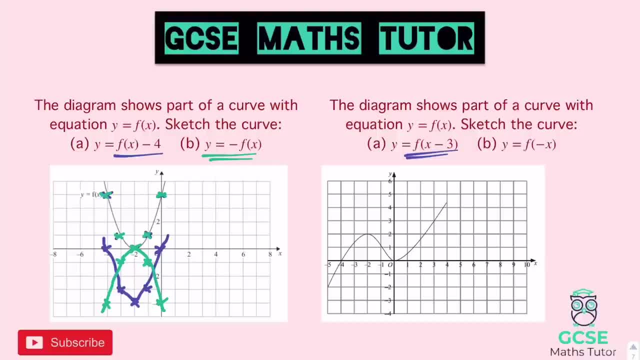 going to affect the x coordinates and it's going to go right 3 or add 3 to all of them. So we've got a few here to move. We've got this one, we've got this one. Let's have a look. This one here. 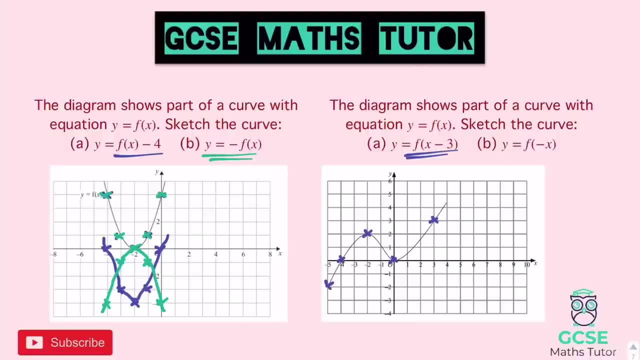 this one here and this one here, and they are all going to go right 3.. So, starting from the right, let's move that right 3, that one right 3, that one right 3.. Let's have a look at the next one. 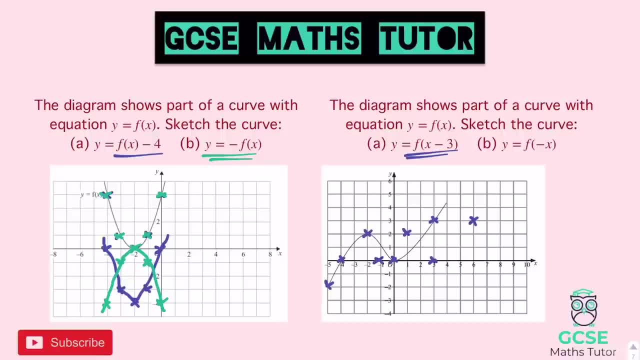 close, Right 3, and where's the last one? Right 3 is there. There we go, And then obviously, just drawing that up as best as you can with a nice smooth curve going through all those coordinates, There we go and there's your little graph transformation there And onto the last one. 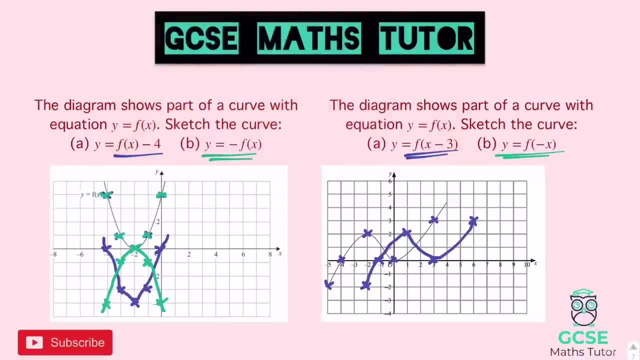 we've got minus x, so changing the x coordinates there, flipping the signs on the x coordinates, So this one here has an x coordinate of 3, and that's going to go to minus 3, which is over here. We've got this one here which is on z. 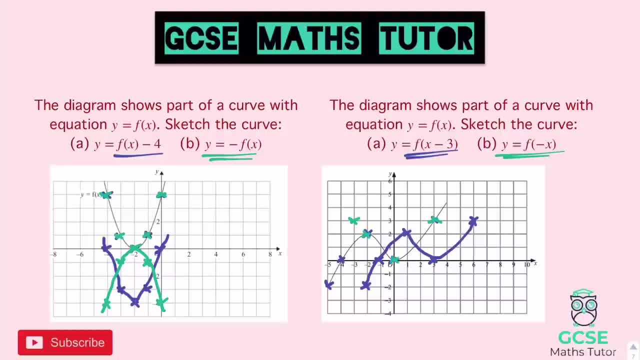 so that's not going to change. We've got minus 2 here, which is going to go to positive 2, which is going to be there. It gets a bit messy on top of each other here, So we've got minus 4,. 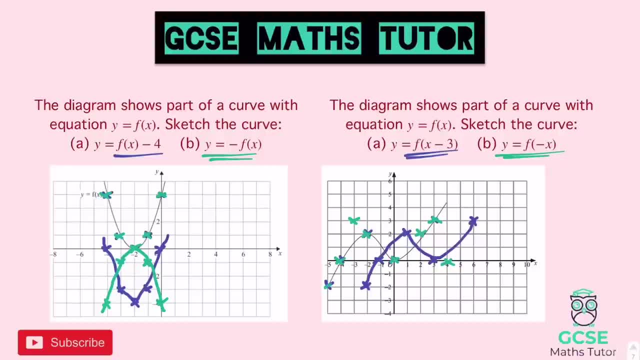 that's going to go to positive 4.. And we've got this one here which is at minus 5, and that's going to go to positive 5.. Right, that is going to be quite difficult for me to draw on top of. 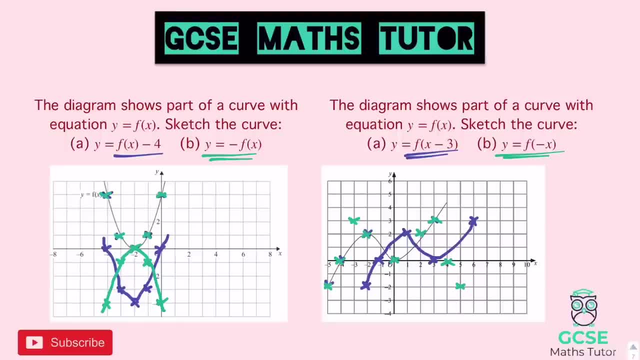 there, Let's think about what this is going to look like. Okay, so as best as I can, Oh, let's start that one again. So that's going to go up through here, down and up, And actually it extends a little bit, so we could extend it a little bit there. 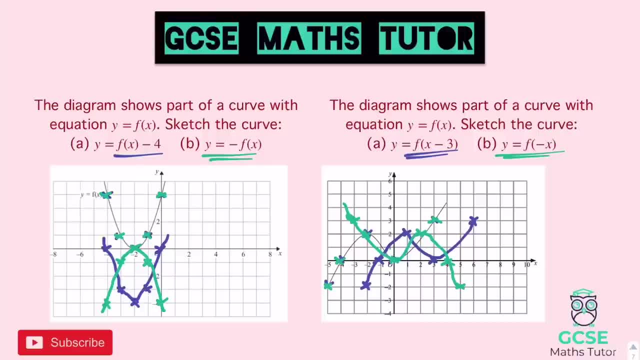 There we go. So it does a reflection there in the y-axis, Okay, so just reflecting it around as best as you can, But obviously you can only do your best there with your sketches. But that hopefully gives you a general idea of what these actual graph transformations actually do to the 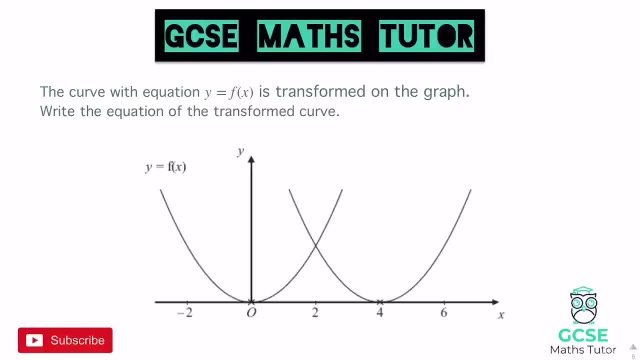 graph. I've got one more for you to have a look at before we finish. Okay, so last question. We've got the curve of the equation f of x is transformed on the graph And here's our equation f of x. so it's this graph on the left. here Write the equation of the transformed curve Now. 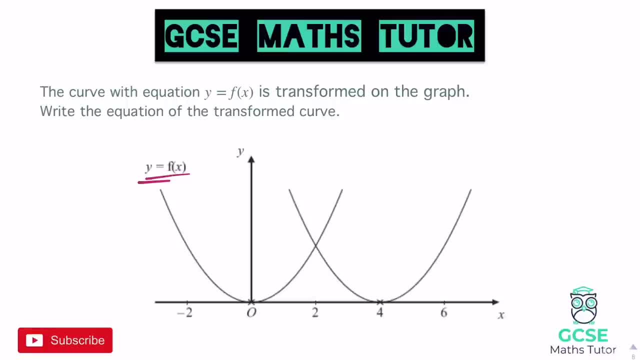 there are so many different ones of these, but it just follows all the rules that we've just looked at before. So this actual graph here, if you have a look. f of x, the points have moved. Okay, so this point here has moved to this point here and that has gone over to the right, Okay. 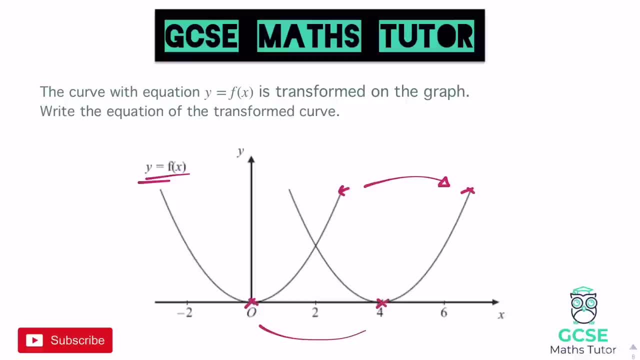 having a look at this point here. it's moved to here And again it's gone over to the right, And the same for the last one. These two points here have moved over to the right. Now what we do is use the number down the bottom for this one. Okay, we can see down here. it goes from 0 to 4.. 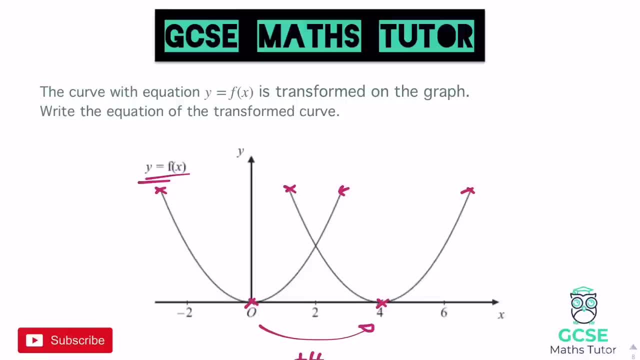 So it has gone right. 4, or 4 has been added to the x-coordinate there. Okay, let's just actually write that a bit higher. There we go. So that has added 4 to the x-coordinate. Now, if we are, 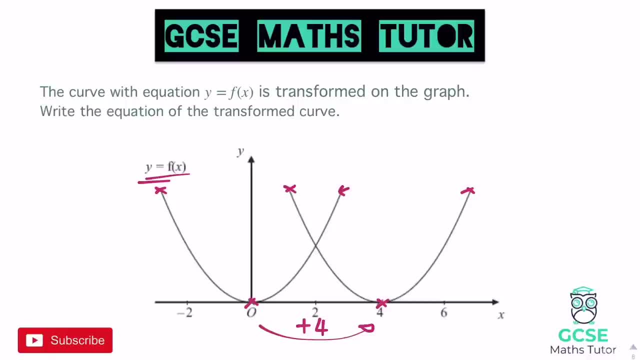 changing the x-coordinate. that means it has to go inside the bracket, doesn't it? So we would have y equals f of, and in the bracket x, And to move right 4 or plus 4, we have to write the. 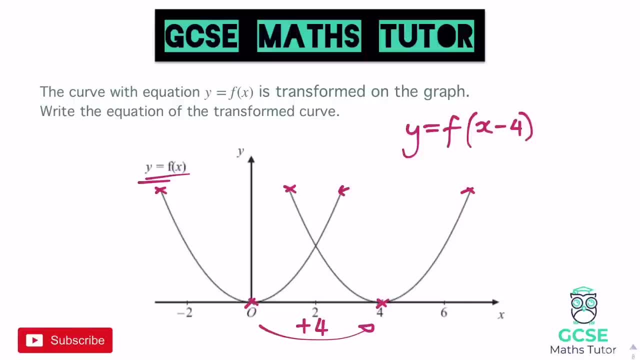 so it would be minus 4.. There we go, And that would be the equation of this curve on the right, And there's obviously so many different ones that you could do here, but all you need to make sure you do on a question like this is find the coordinates, see what's happened to them. 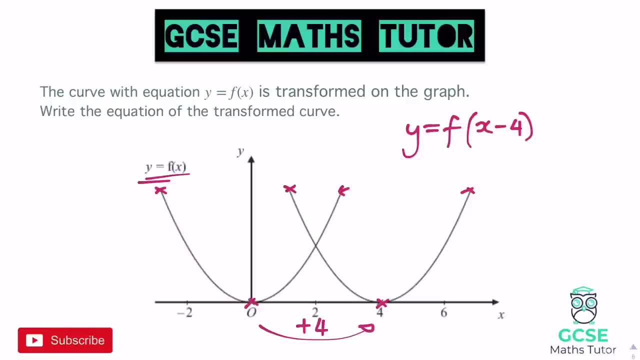 and obviously just relate that and correspond it back to our little table there. Has the x-coordinate changed, in which case it's in the bracket. Have the y-coordinates changed, in which case they're going to be outside the bracket? Okay, the only thing you need to be careful of is when it's a 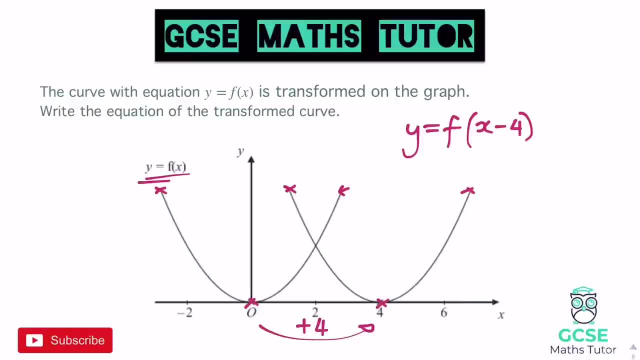 reflection. just making sure that you are careful there, because it's a little bit of an opposite inside the bracket: a minus inside the bracket does a reflection in the y-axes and a minus outside the bracket does a reflection in the x-axes, but it changes the corresponding coordinates. So 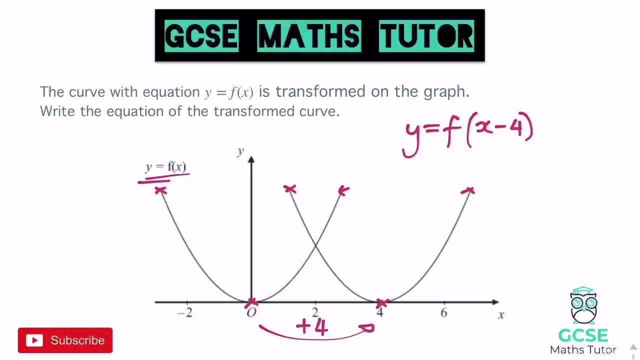 inside the bracket with a minus changes the x-coordinates, which does a reflection in y, and outside the bracket changes the y-coordinates but ends up doing a reflection in x. But there is just one little question there to be thinking about and how you would apply this okay. 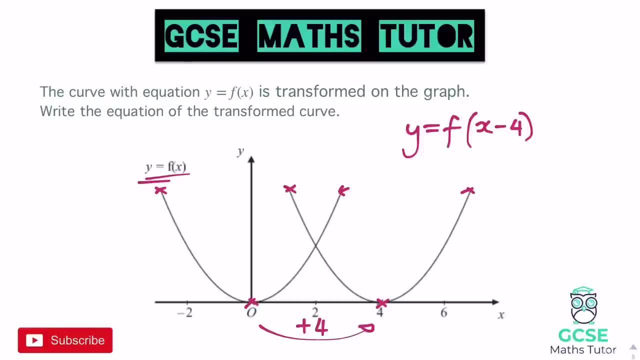 if you did have to write the equation of the transformed curve or graph or whatever it is that you have to do. But there we go. a bit of an overview on transformation of graphs. Hopefully you found that useful. If it was helpful, please like, please comment, please subscribe. and I'll see you for the next one.